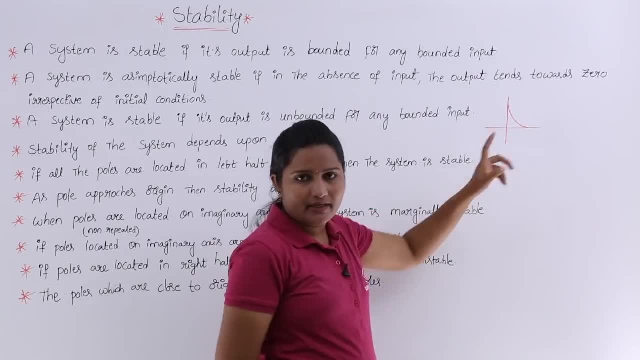 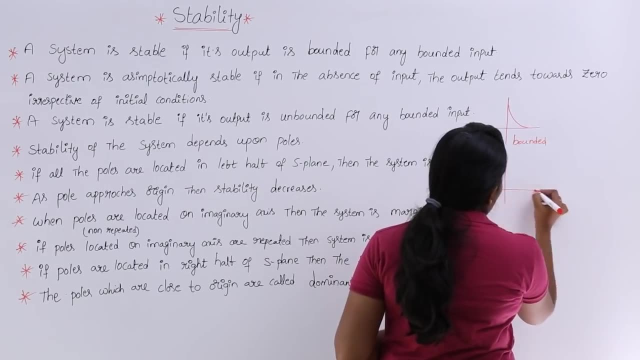 minima is 0.. So these two are finite. so we can say: this is a bounded signal. so this is bounded signal, For example, if you are having ramp. So if you are having ramp, So the minimum value. 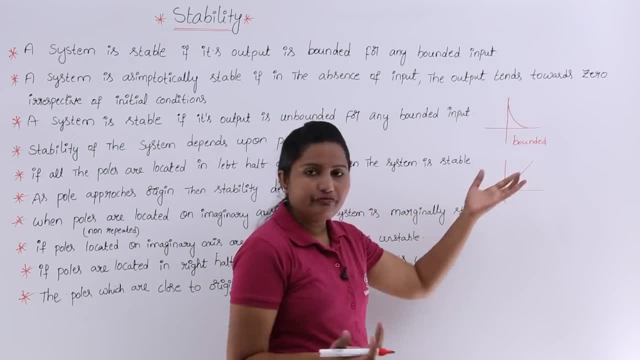 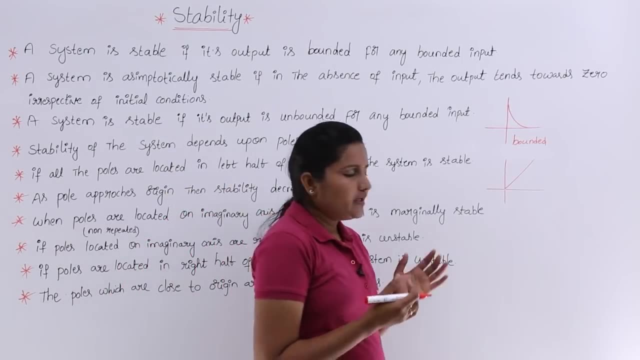 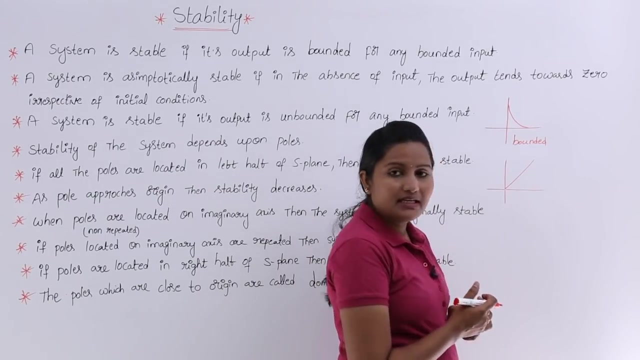 of ramp is 0 volts and maximum- we do not know at t is equivalent to infinity. you will get some infinity. So here the maximum value is not finite, only minimum value is finite. In this case the signal is said to be unbounded. So this is unbounded signal Coming to a 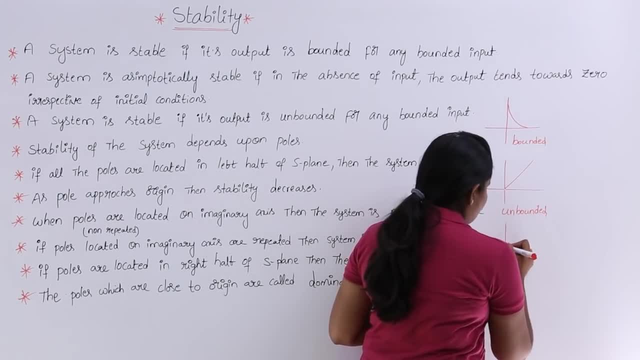 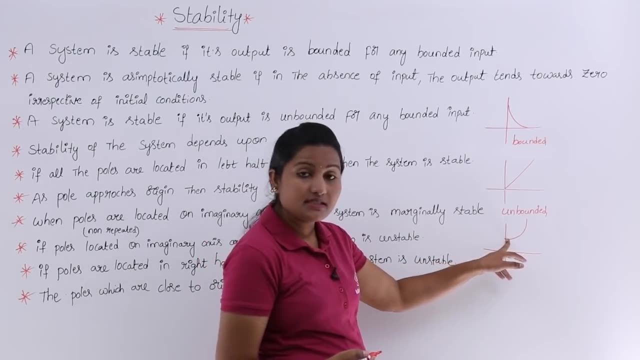 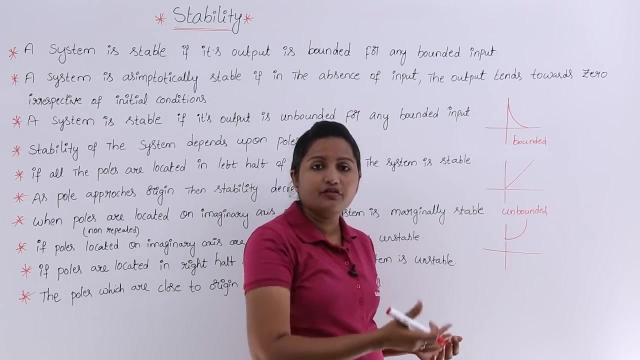 bounded signal. So this is a bounded signal. So this is a bounded signal. So this is a bounded signal. Coming to another signal like this: if you are having signal like this, the minimum amplitude is finite, but the maxima amplitude- we do not know this- is this- is continuously exploding. 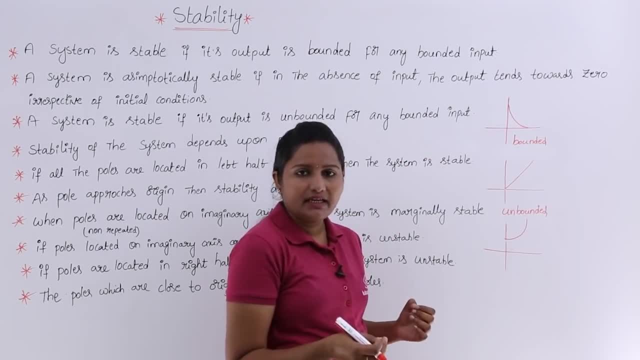 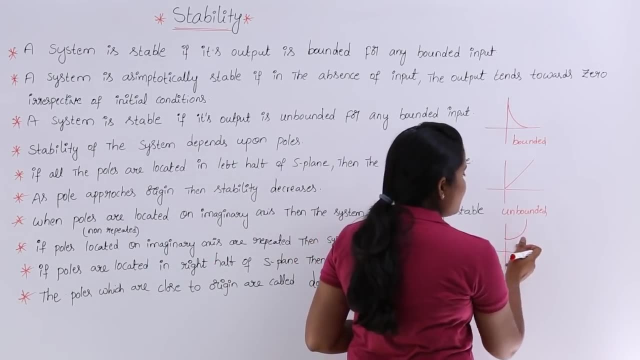 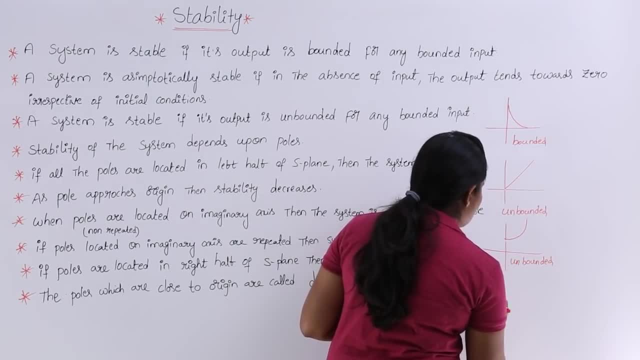 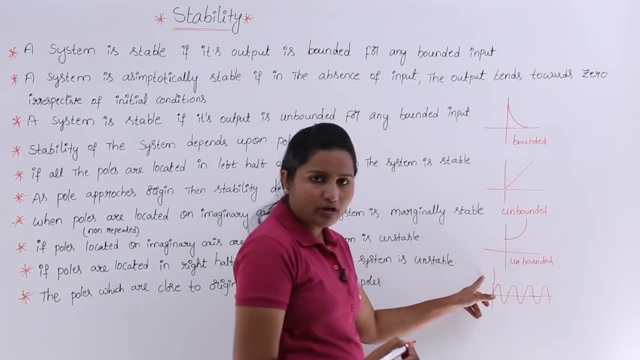 Coming to some sinusoidal form of signal. So like this, if you are having like this, So here the maximum may be 1 or 2 or anything. maximum is finite, minimum is 0 or minimum is negative value. So if this is fixed to a reference value, if it is fixed to a offset, 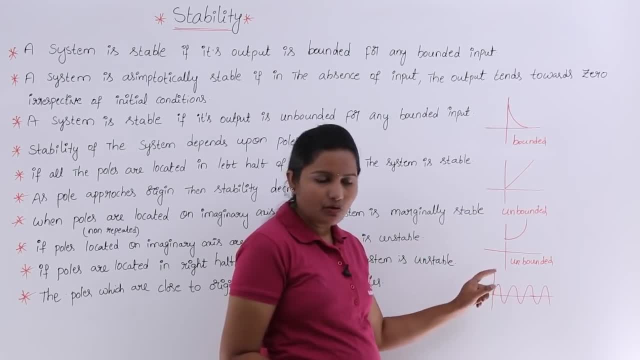 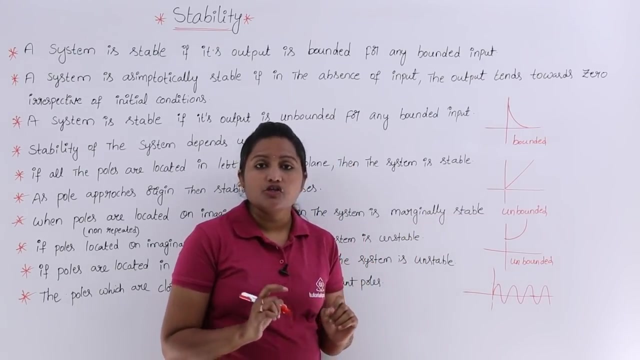 then we can say: maximum is some value, minimum is 0. But here you are having two sided signal. minimum is some minus 1, for example, maximum is plus 1. Here, whatever the amplitudes of this signal is there, those amplitudes are finite. So we can say: this is also bounded. 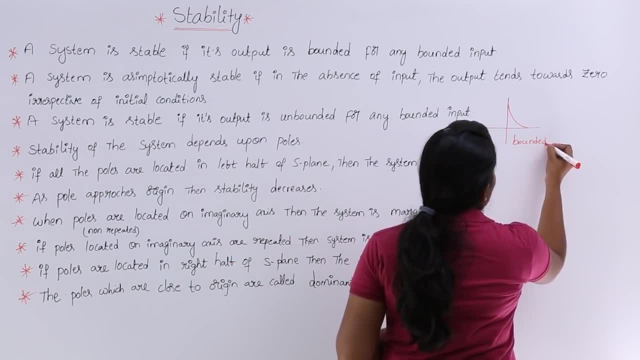 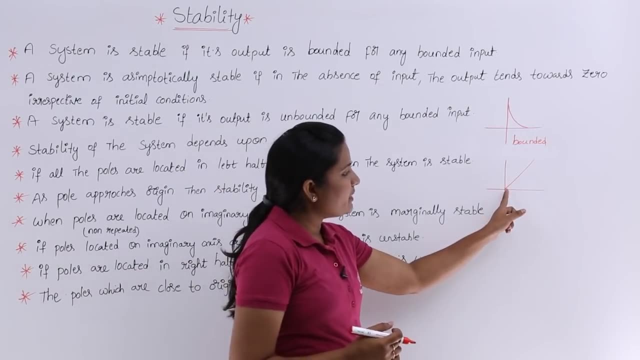 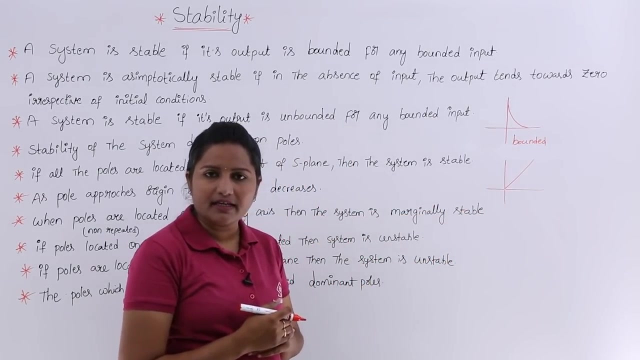 is a bounded signal, so this is bounded signal. for example, If you are having ramp. so if you are having ramp, so the minimum value of ramp is 0 volts and maximum- we don't know- at t is equivalent to infinity. you will get some infinity, so 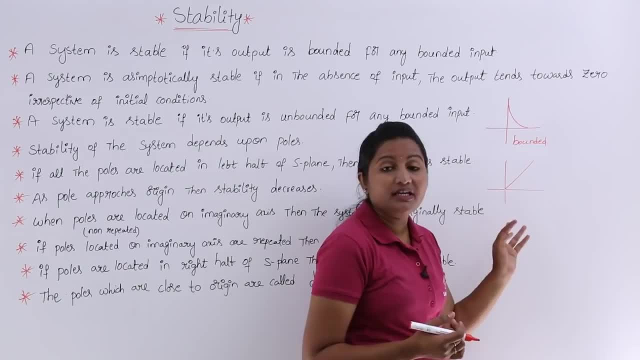 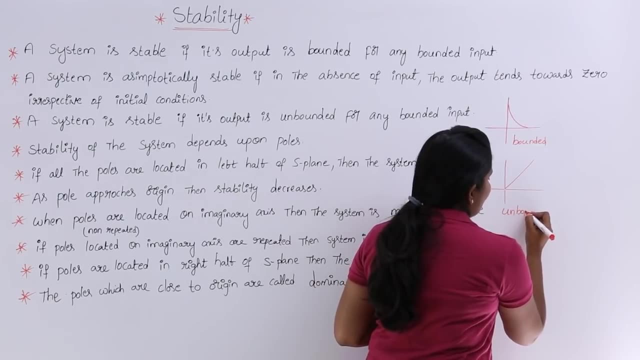 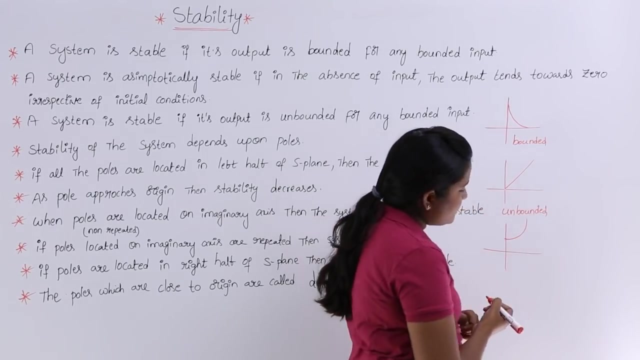 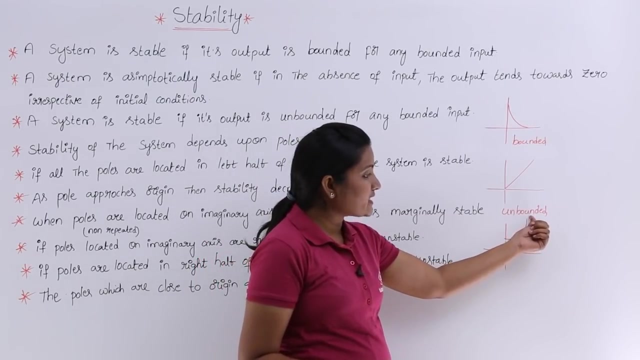 here the maximum value is not finite, only minimum value is finite. in this case, the signal is said to be unbounded. so this is unbounded signal. Now, if you are going to another signal like this, if you are having signal like this, the minimum amplitude is finite, but the maxima amplitude- we don't know this is this- is continuously. 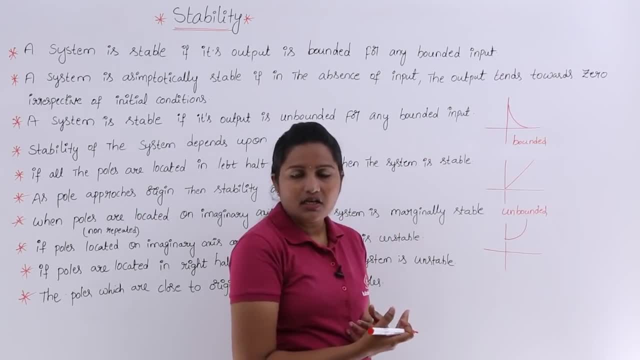 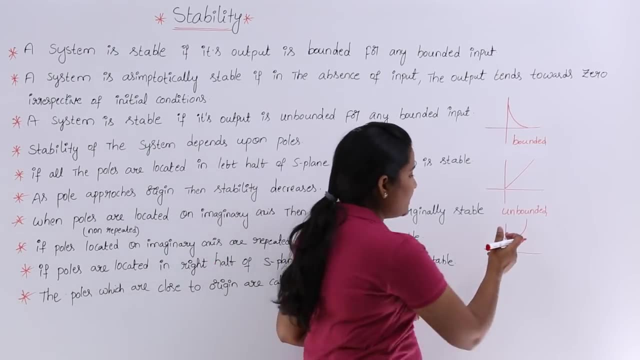 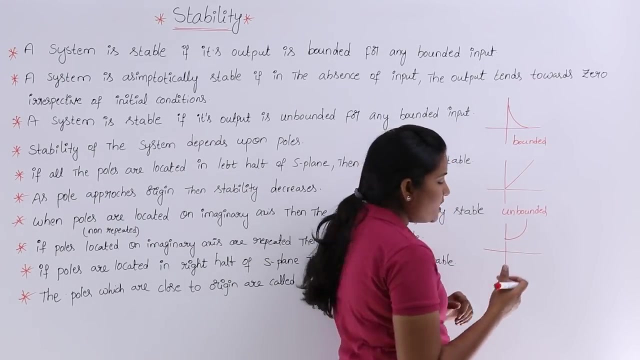 exploding, continuously rising signals. so generally continuously rising signals are said to be unbounded signals. so here, here also, we can't trace the maxima and minima, so we can't trace the maximum amplitude of the signal. at t is equivalent to infinity. so we can say this: 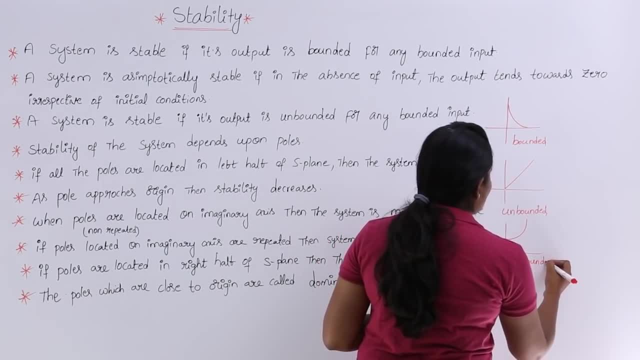 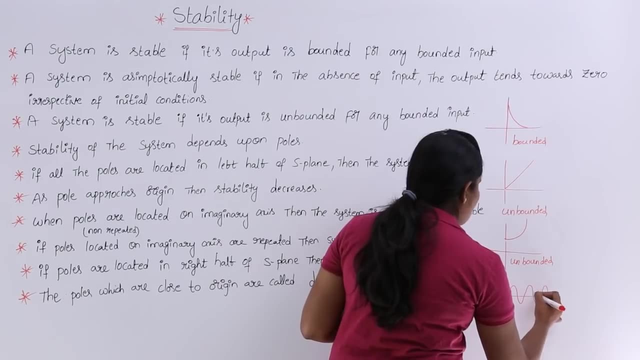 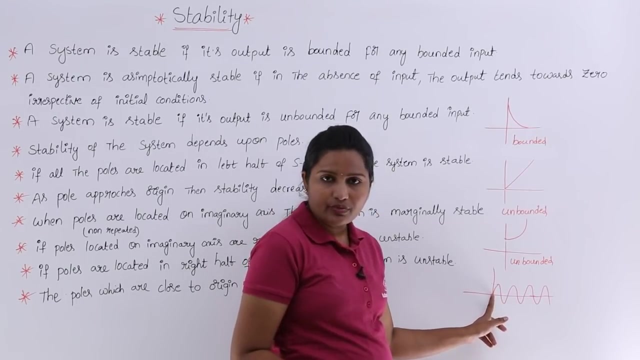 is also unbounded, Coming to some sinusoidal form of signal. so like this, if you are having like this, so here the maxima may be 1 or 2 or anything. maxima is finite, minima is 0 or minima is negative value. 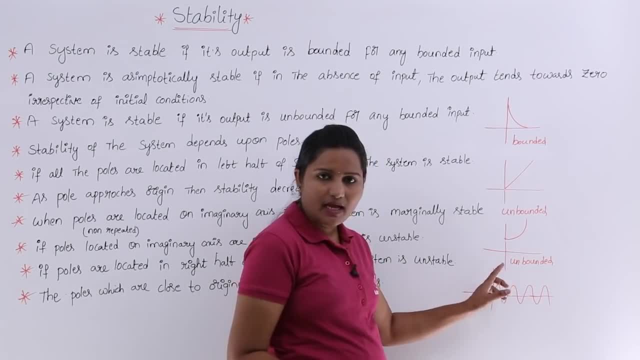 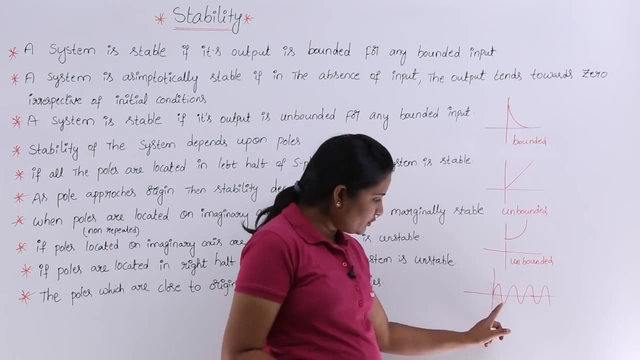 So if this is fixed to a reference value, if it is fixed to a reference value, if it is fixed to a offset, then we can say: maximum is some value, minimum is 0, but here you are having two sided signal. minimum is some minus 1, for example, maximum is plus 1 here, whatever. 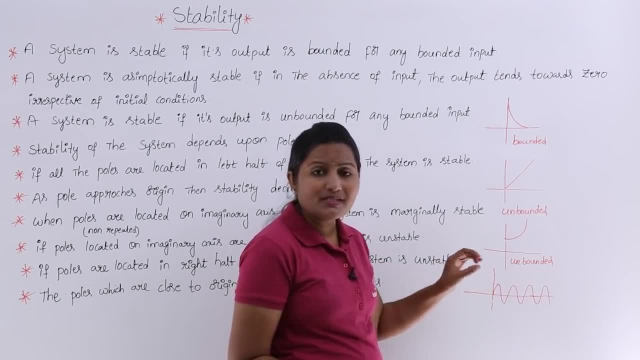 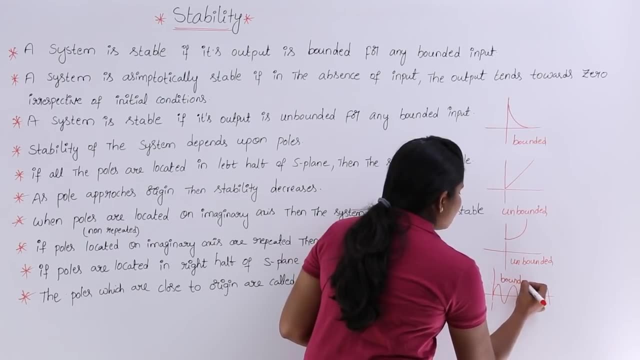 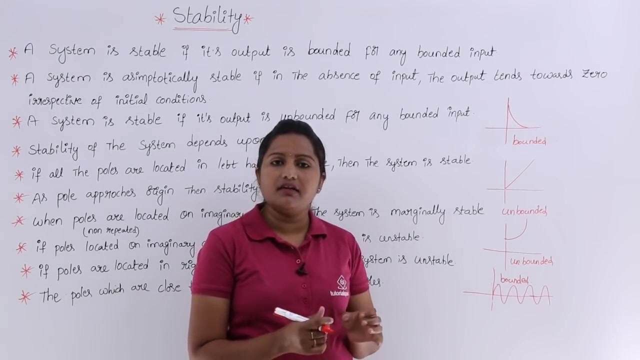 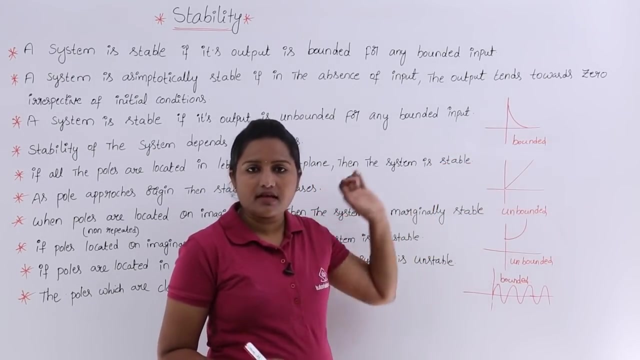 the amplitude of this signal is there. those amplitude are finite, so we can say this is also bounded signal. so the signals in the continuously rising form are said to be unbounded. remaining signal which are having finite maxima minima are said to be bounded. So continuously rising signals are unbounded. 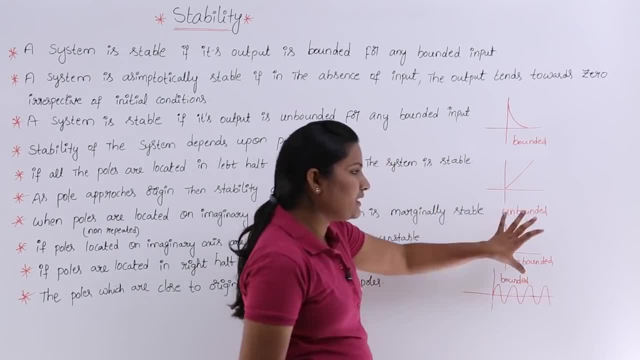 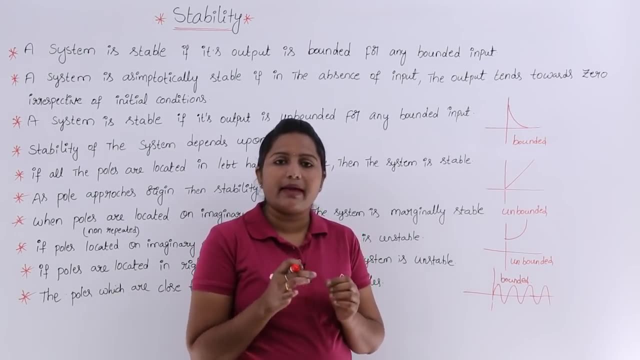 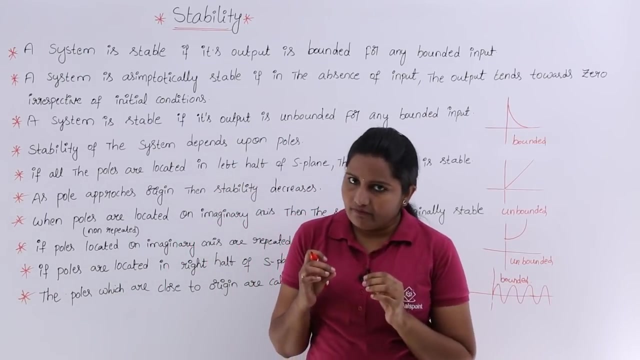 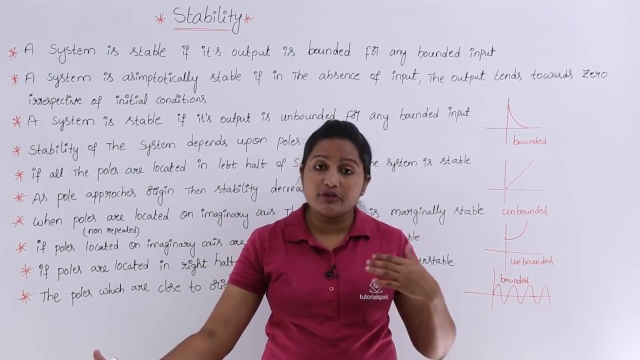 signal. So the signals in the continuously rising form are said to be unbounded. remaining signal, which are having finite maxima, minima are said to be bounded, So continuously rising signals are unbounded. So when you given a bounded signal as input, if you are getting unbounded signal, that means 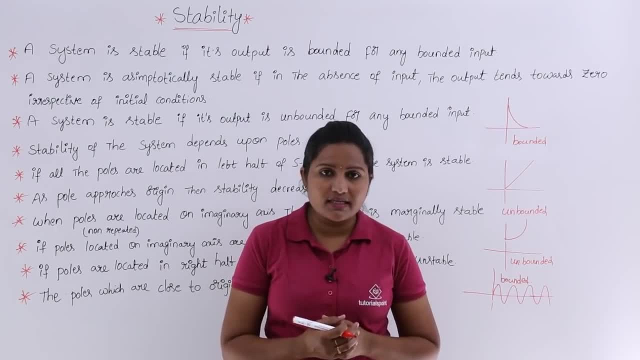 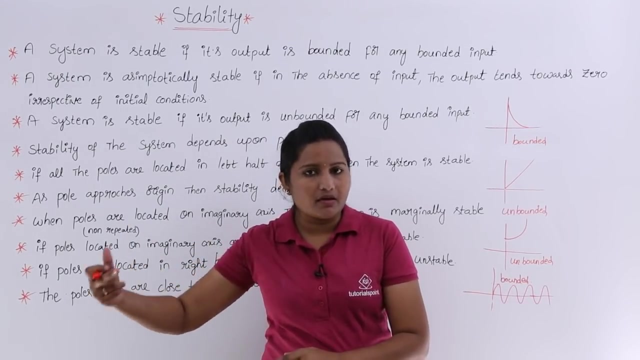 your maxima or minima may be infinite, then you can say this system is unstable system. Then what is the condition for stability means? So, if the system is stable, if you given bounded signal, you need to get the bounded signal as output. If you are getting unbounded output, 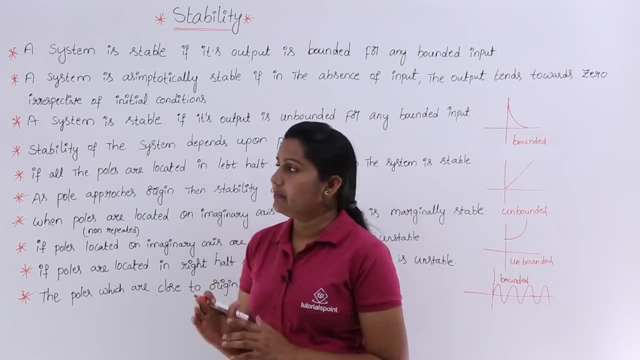 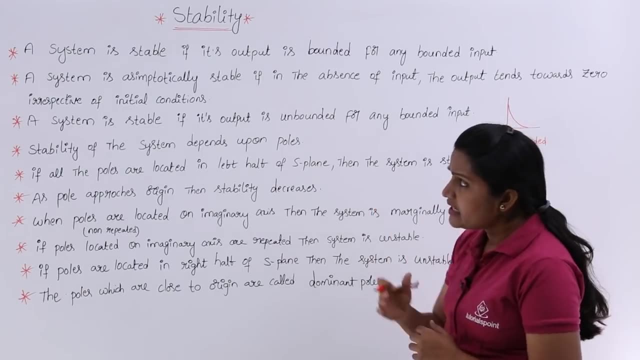 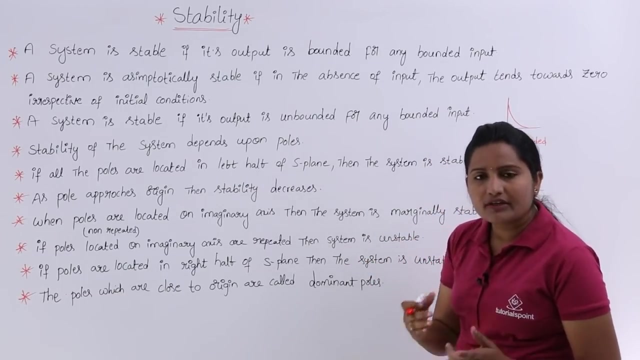 for bounded input. ok, then that system is unstable. So this is the first point: a system is stable if its output is bounded for any bounded input. Next, a very important point is: a system is asymptotically stable if, in the absence of input, if the output is tending to 0, apart from the initial conditions. 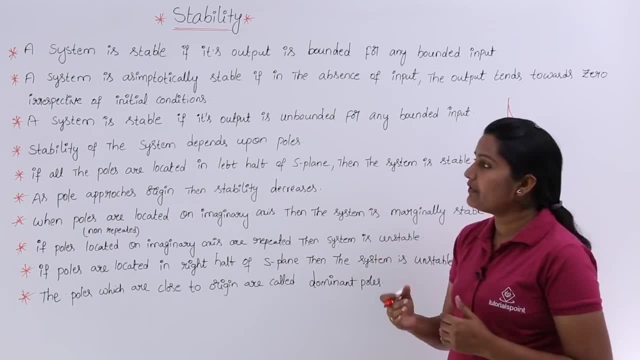 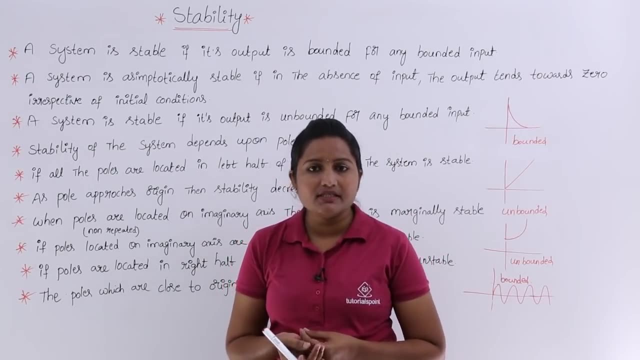 irrespective of the initial conditions, then we can say that is asymptotically stable system. When we can say a system is asymptotically stable system means in the absence of input, without giving input, the system is producing some response which is tending to 0, irrespective. 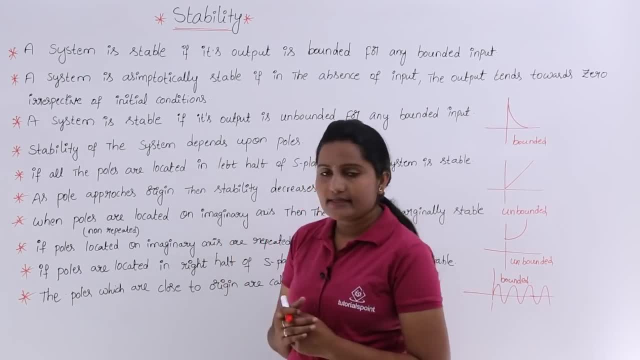 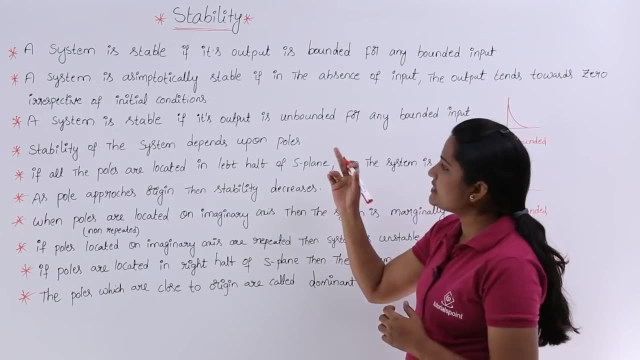 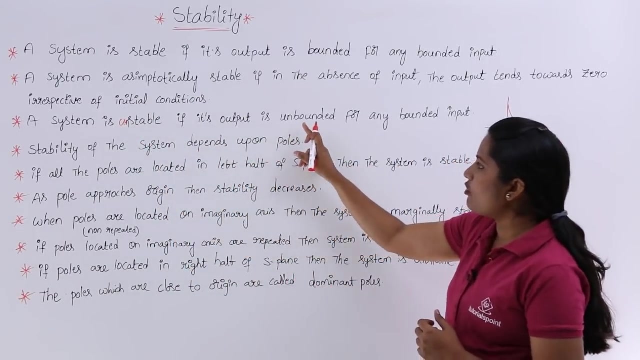 of the initial conditions, or called, is called as asymptotically stable system. Now, coming to the third point, a system is stable if its output is unbounded. So this is a system is unstable. A system is unstable If its output is unbounded for any bounded input. So this is the definition for unstable. 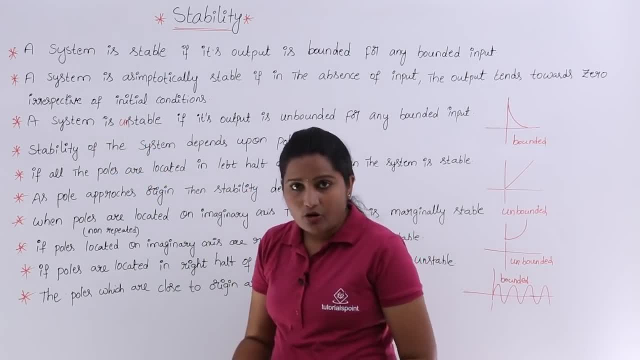 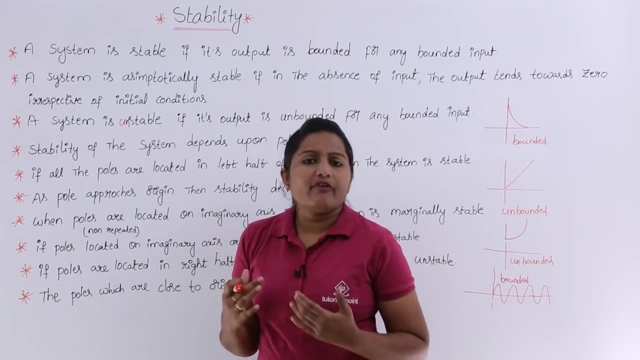 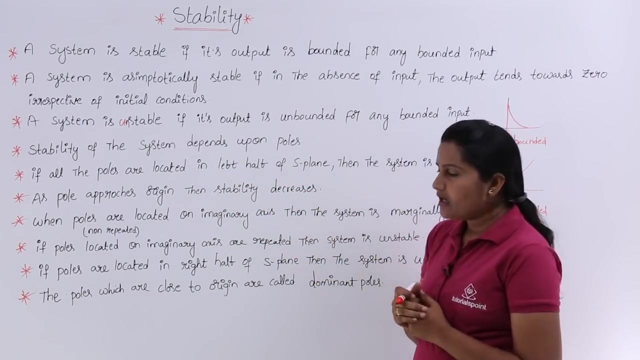 system. A system is unstable if its output is unbounded for a bounded input Coming to the poles. poles will define the stability. If all the poles are located in the left half of S plane, then the system is stable. Stability of the system depends upon: 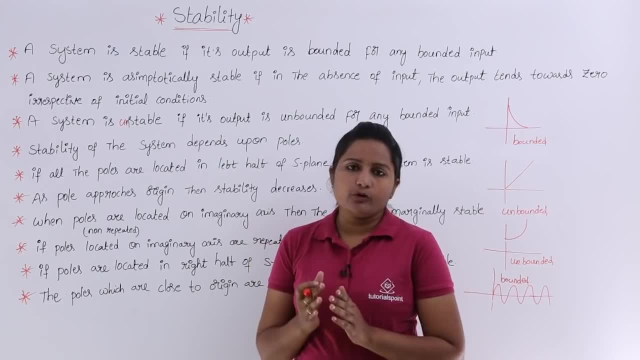 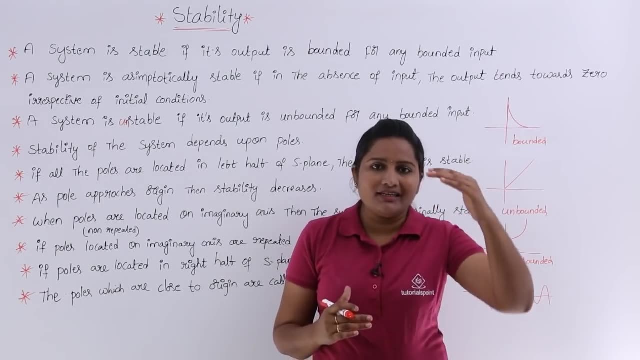 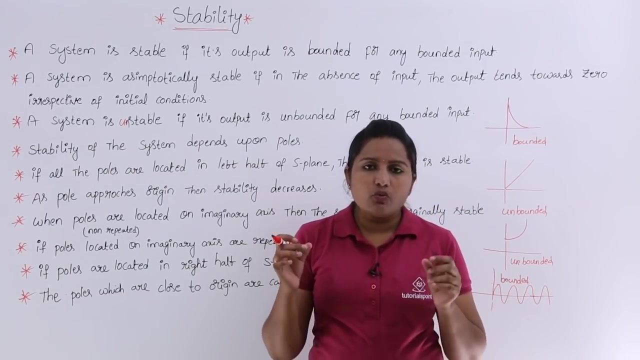 the poles of transfer function. So what is meant by poles? What is meant by zeros? You already know about poles and zeros If you are having some transfer function in A by B form. So the numerator indicates zeros and denominator indicates poles. So whatever the poles location, is there that? 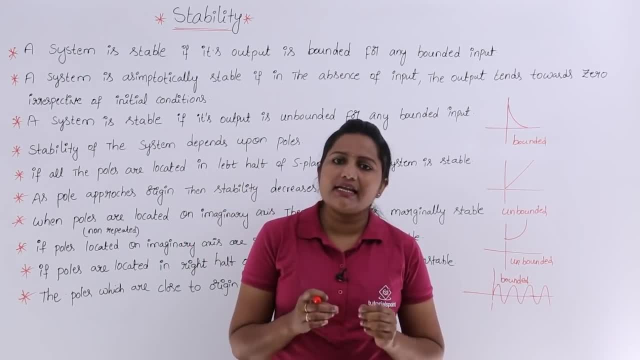 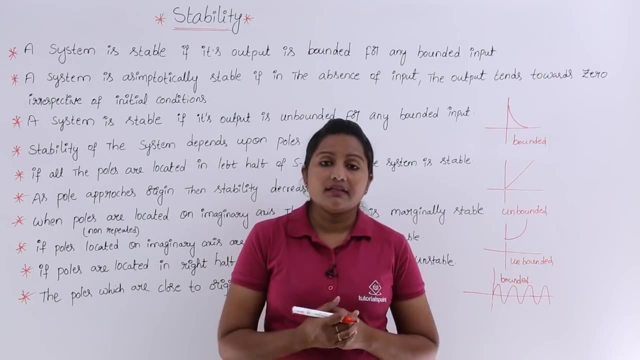 So when you given a bounded signal as input, if you are getting unbounded signal, that means your maxima or minima may be infinite, then you can say this system is unstable system. then what is the condition for stability means? so if the system is stable, if you given bounded, 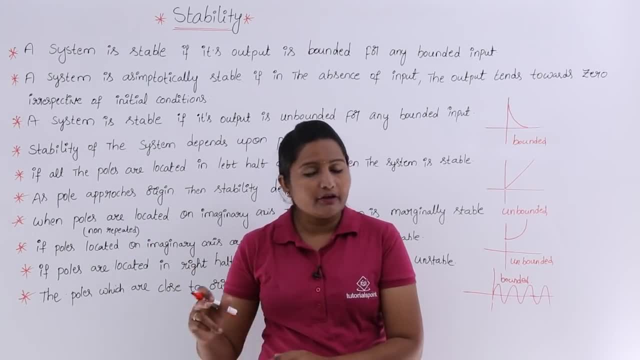 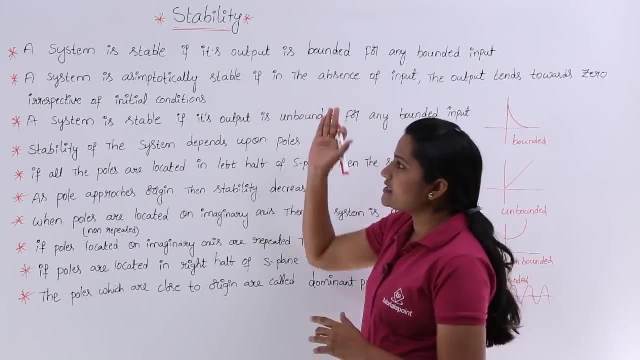 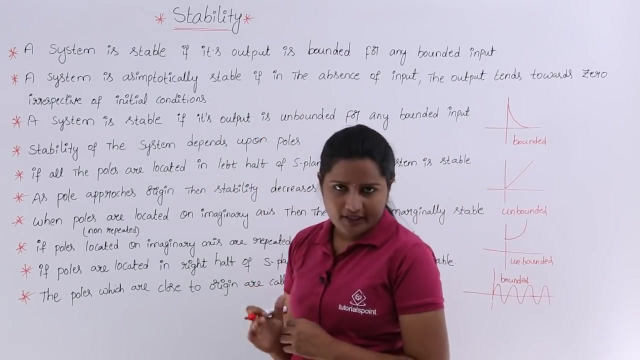 signal, you need to get the bounded signal as output. If you are getting unbounded output for bounded input, then that system is unstable. So this is the first point: a system is stable if it is output is bounded for any bounded input. Next, a very important point is: a system is asymptotically stable if, in the absence of 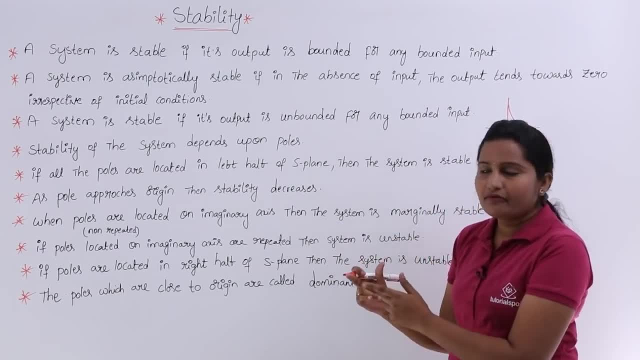 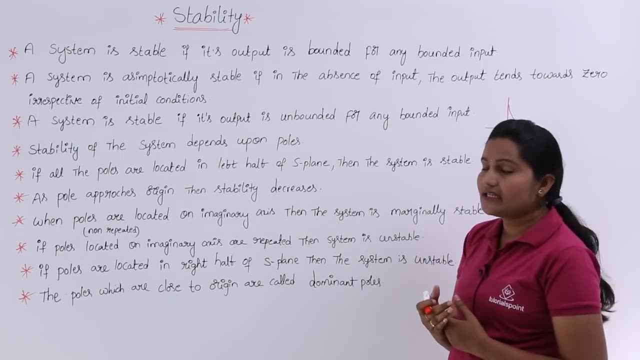 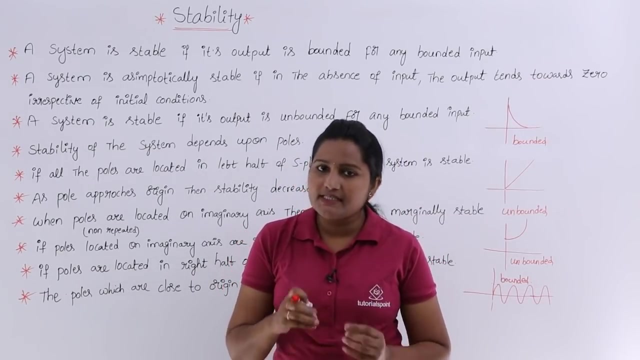 input. if the output is tending to 0 apart from the initial conditions, irrespective of the initial conditions, then we can say that is asymptotically stable system. When we can say a system is asymptotically stable system means in the absence of input, without giving input, this system is producing some response which is tending to 0, irrespective. 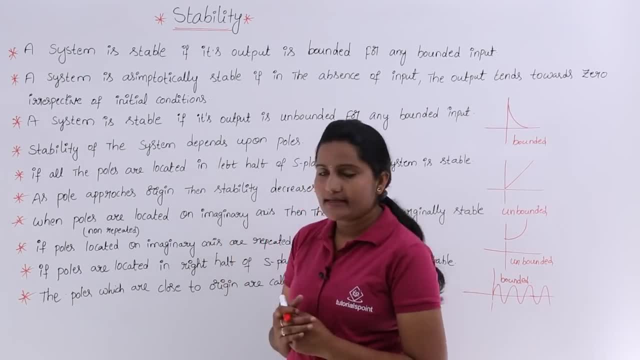 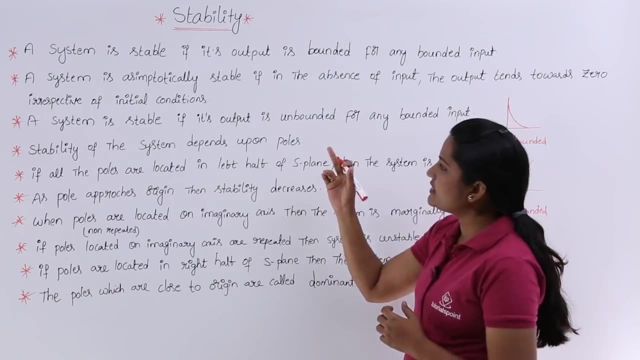 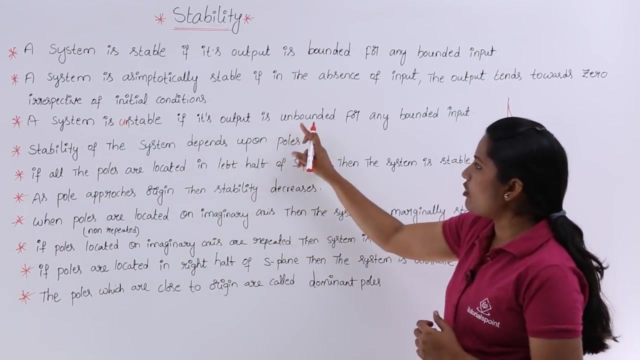 of the initial conditions, or called, is called as asymptotically stable system. Now, coming to the third point, a system is stable If its output is unbounded. so this is a system is unstable. a system is unstable if its output is unbounded for any bounded input. 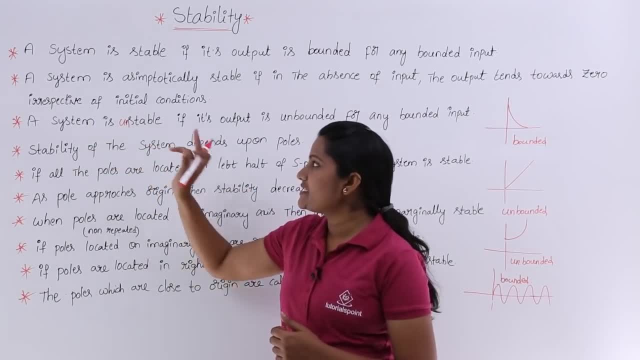 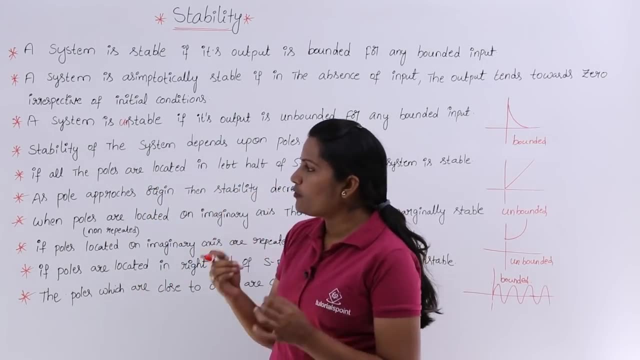 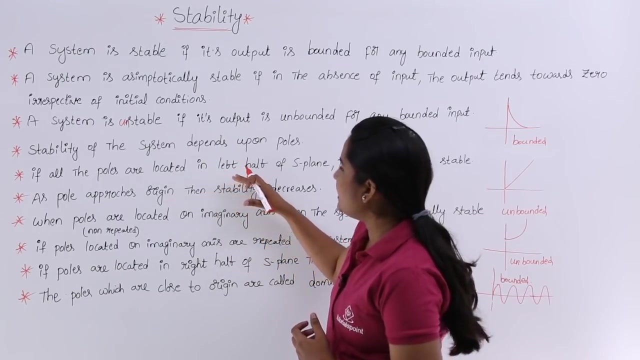 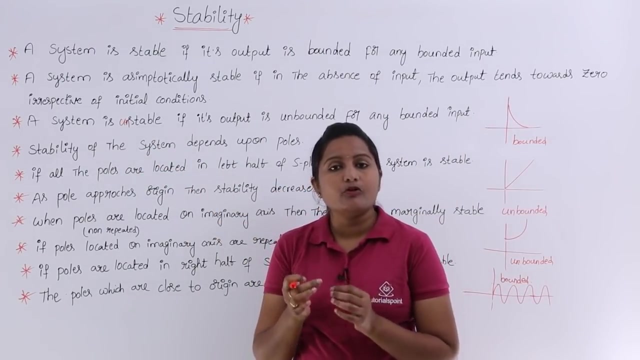 So this is the definition for unstable system. a system is unstable if its output is unbounded for a bounded input Coming to the poles. poles will define the stability. if all the poles are located in the left half of s plane, Then this system is stable. stability of the system depends upon the poles of transfer function. 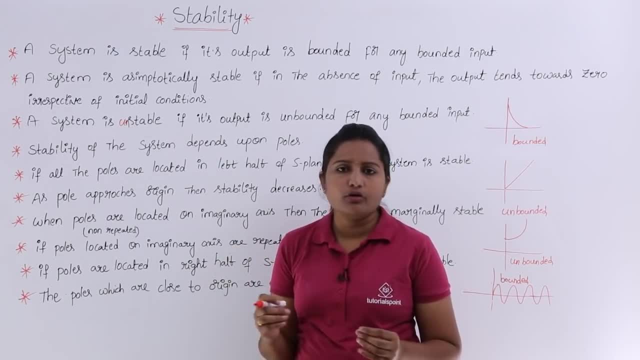 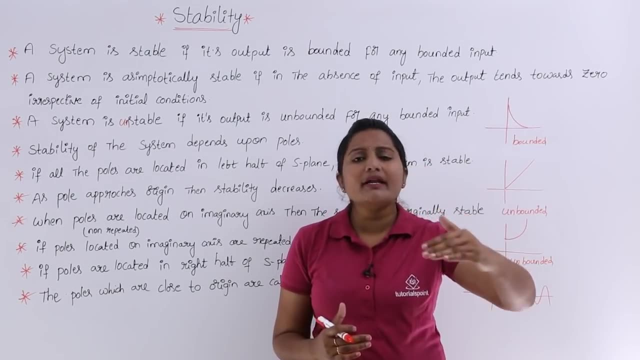 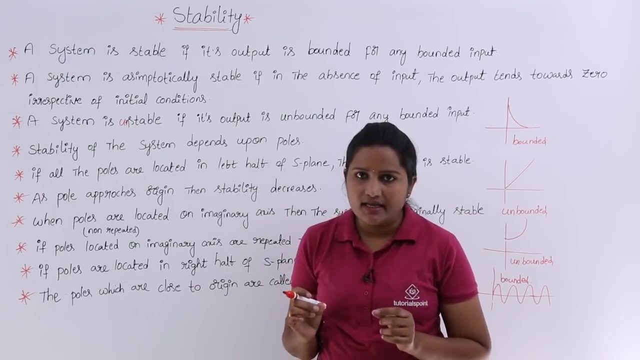 So what is meant by poles? what is meant by 0s? you already know about poles and 0s If you are having some transfer function in a by b form. so the numerator indicates 0s and denominator indicates poles. So whatever the poles location is there, that poles will defines the stability. 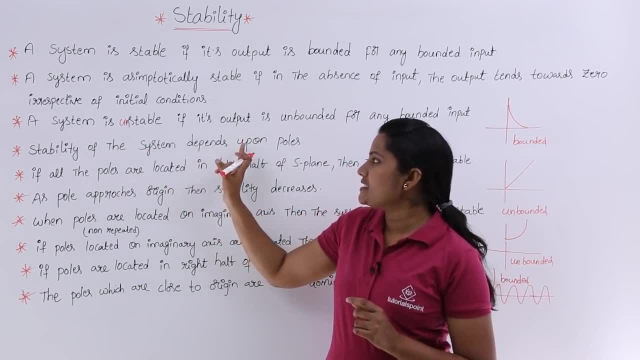 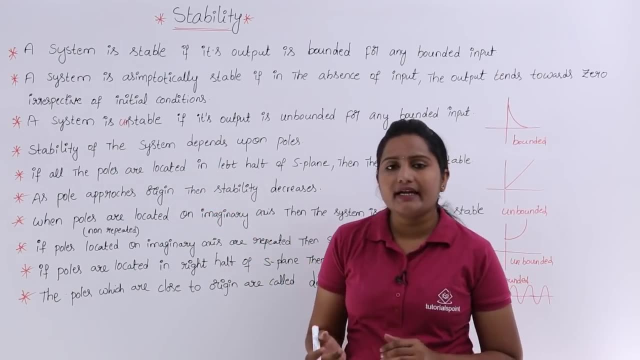 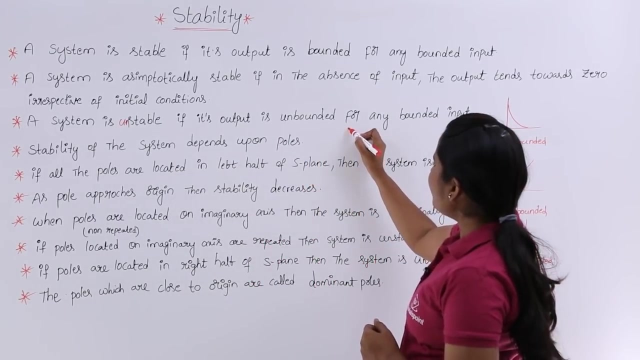 poles will define the stability. Stability of the system depends upon the poles. How that is dependent upon the poles means If all the poles are located in left half of S plane, then the system is said to be stable. For example, if you are having S plane like 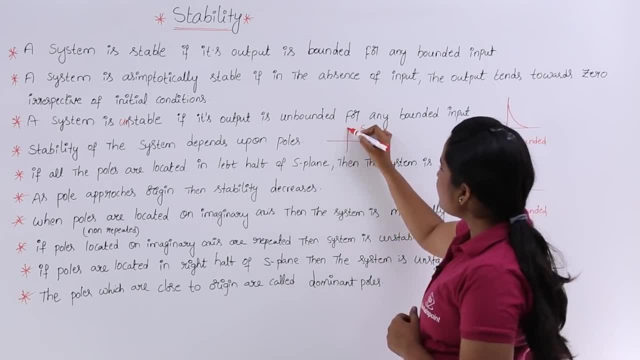 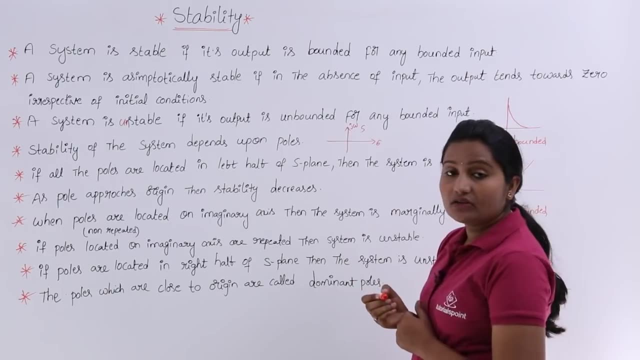 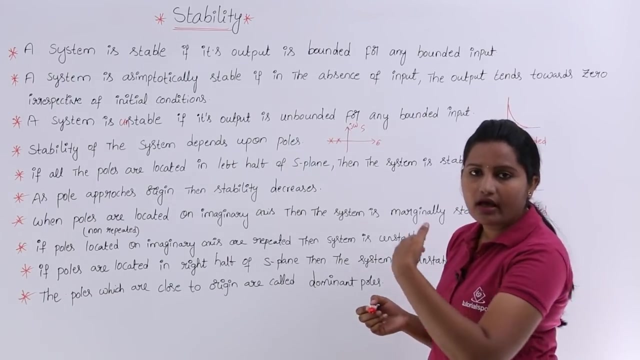 this. So this is total s plane, This is j omega axis and this is real axis sigma. So if all poles located on the left half of S plane means So this side, if you are having two poles, that two poles are located on left half of S plane, Then you can say the left. 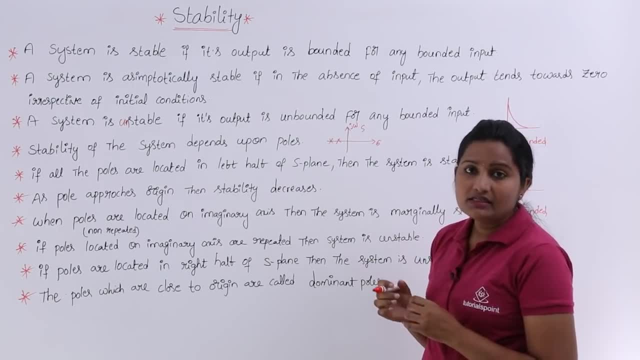 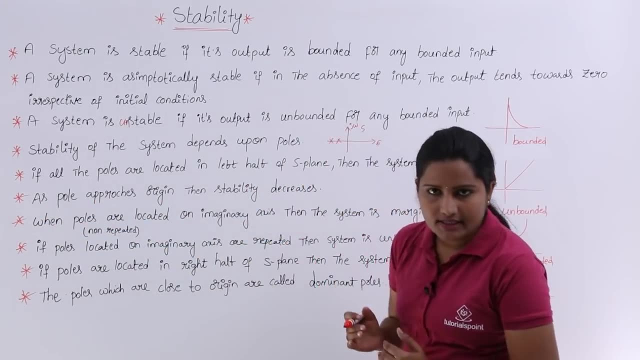 half of S plane is stable. So this is the total S plane. If all poles located in this left half of S plane, If all poles are located in the left half of the S plane, then you can. that is a stable system. then, coming to another point, as pole approaches origin, if pole approaches, 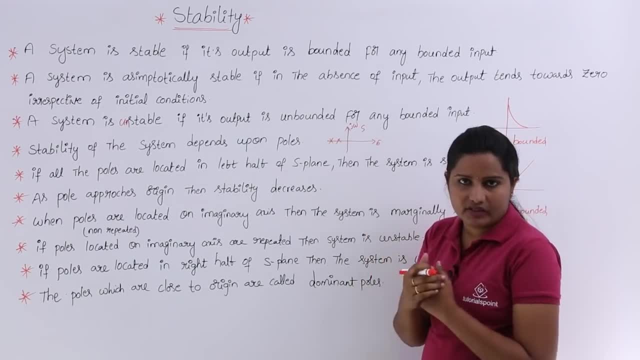 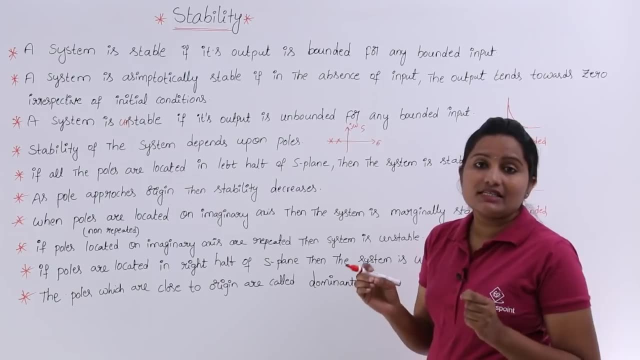 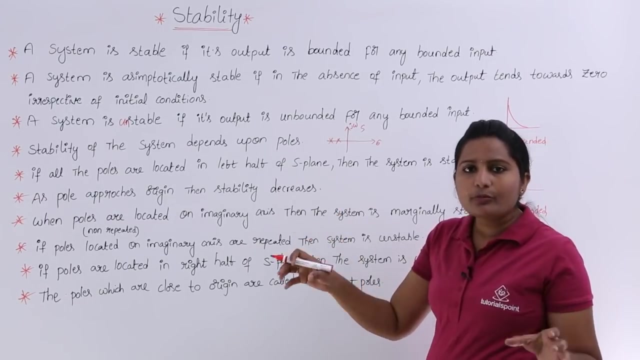 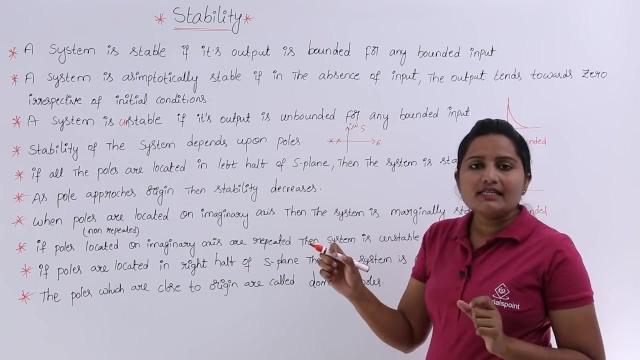 origin, the stability of the system will decrease. so, for example, according to pole zero plot we can say the stability of the system. for example, if you are having two pole zero plots, two pole plots of two systems, by saying that pole zero plot of the systems you can say which system. 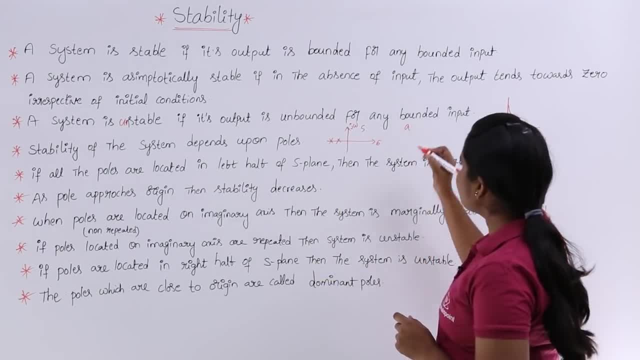 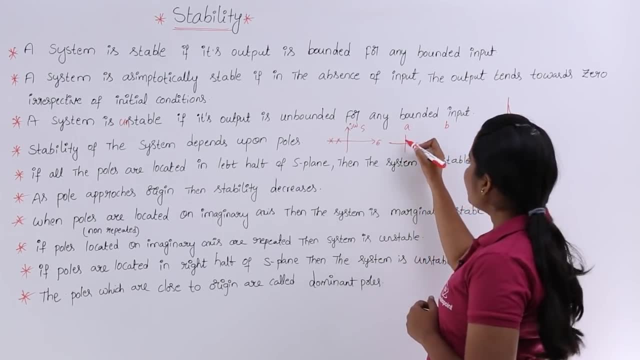 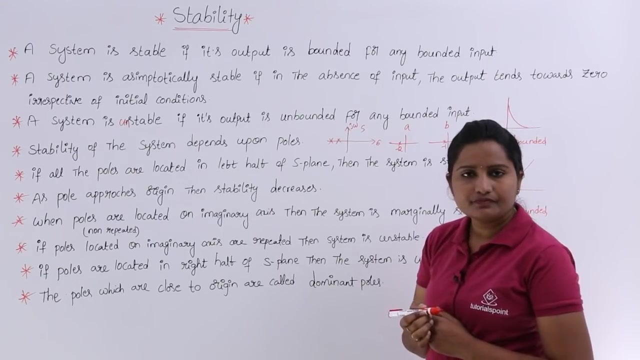 is much stable. for example, i am having system a and i am having system b. i got my pole zero plot. so here at minus two i am having pole and here at minus one i am having pole. for system a i am having pole, only one pole at minus 2, and for system B I am having single pole at minus 1, for example. 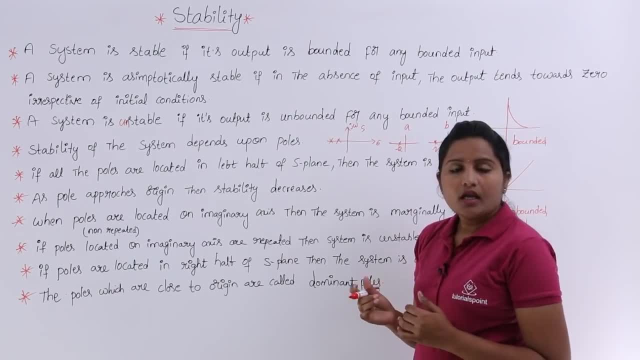 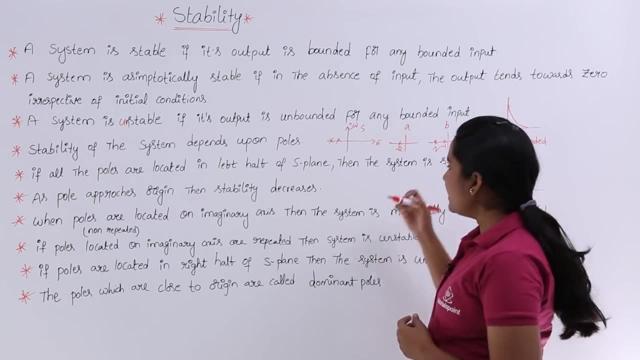 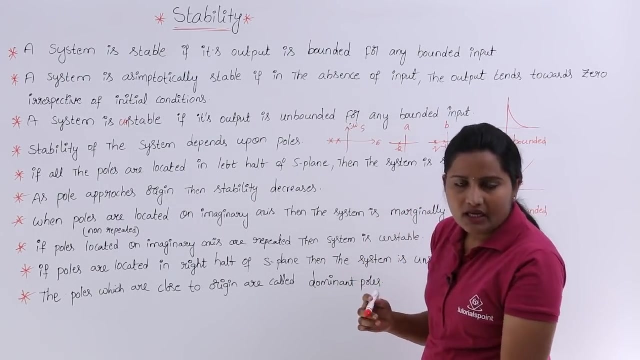 here you are having minus 2 here. which system is much stable means so this system is much stable. why? because here the poles are approaching origin. the poles of system B is very near to origin. if the poles are approaching to origin, the stability of the system will decrease. 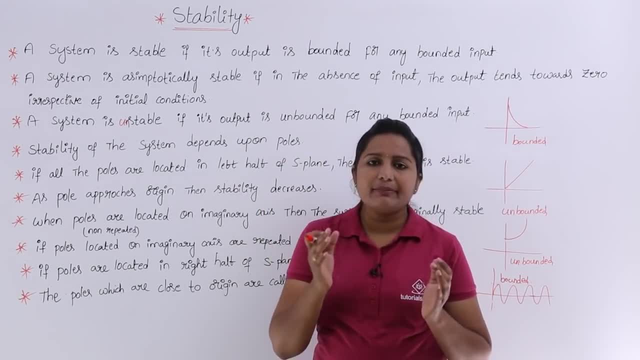 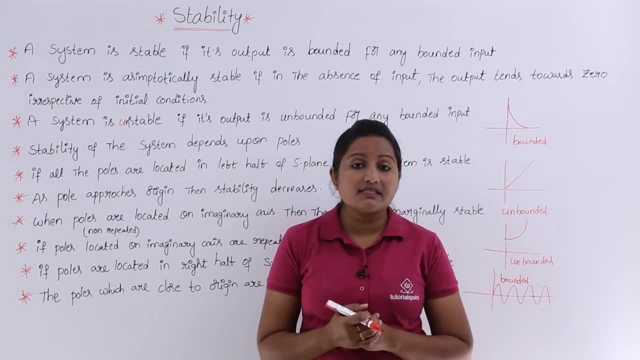 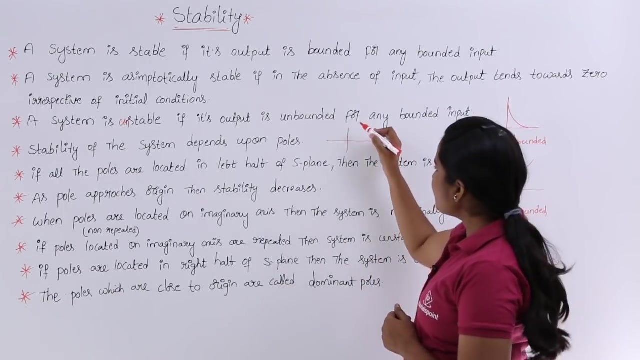 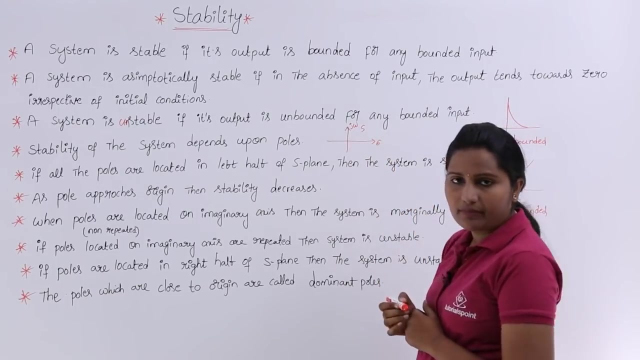 Stability of the system depends upon the poles. How that is dependent upon the poles means if all the poles are located in left half of s plane, then the system is said to be stable. For example, if you are having s plane like this, So this is total s plane. this is j omega axis and this is real axis sigma. 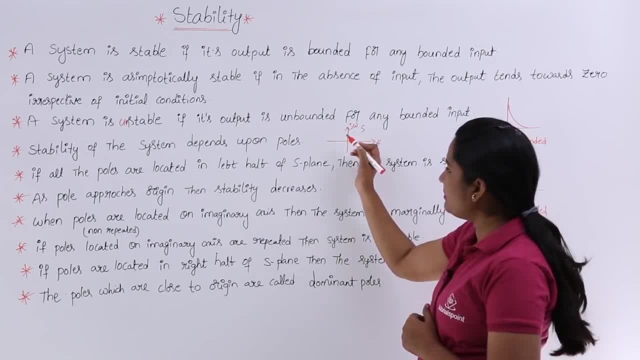 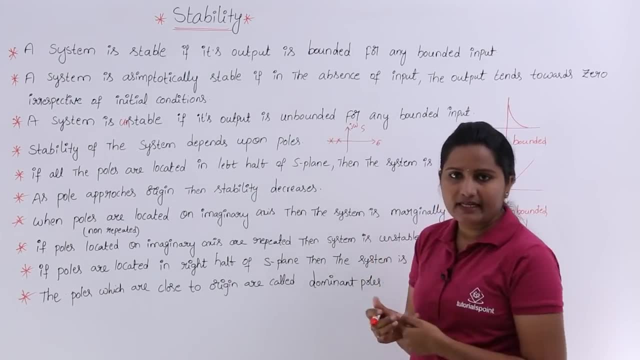 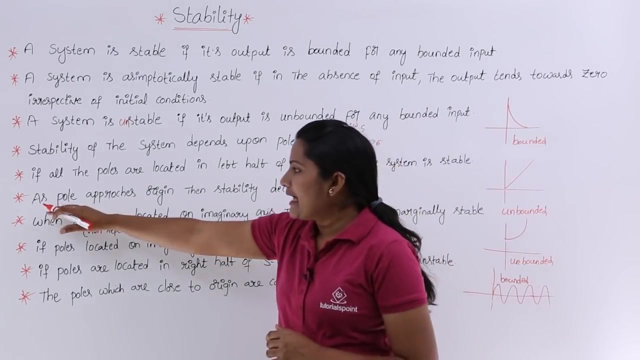 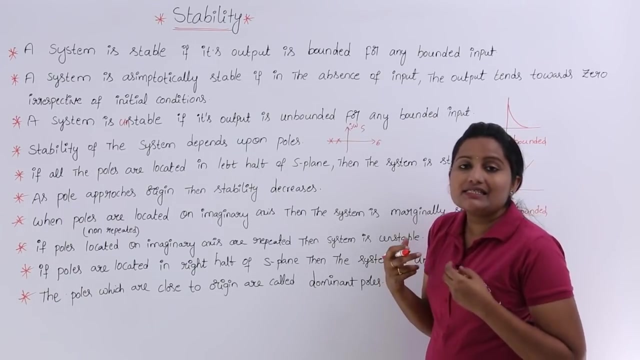 So if all poles located on the left half of s plane means so this side, if you are having 2 poles, Then those 2 poles are located on left half of s plane. then you can say that is a stable system. Then, coming to another point, as pole approaches origin, if pole approaches origin, the stability 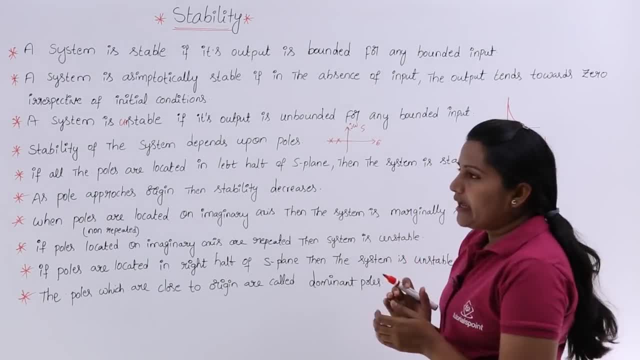 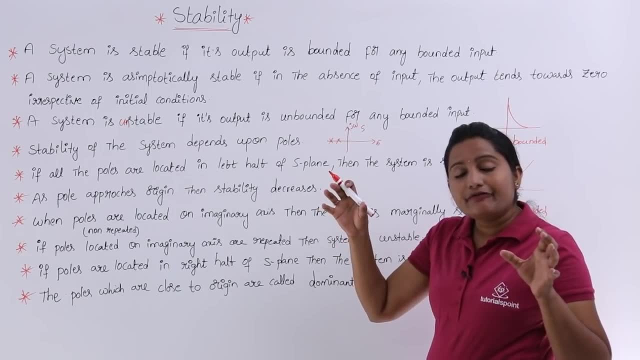 of the system will decrease. So, for example, according to pole zeros plot, we can say the stability of the system. For example, if you are having, recall, two poles which are located under this axis six times, if you are having two pole zero plots, two pole plots of two systems, by saying that pole. 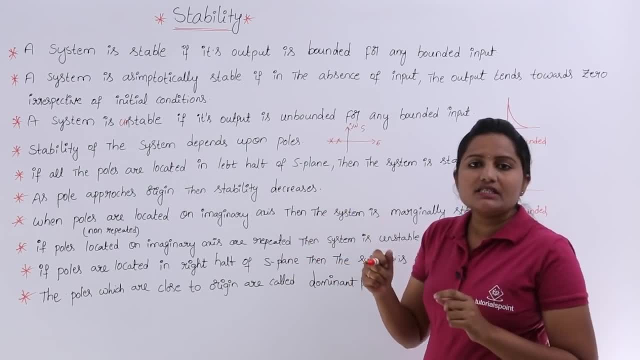 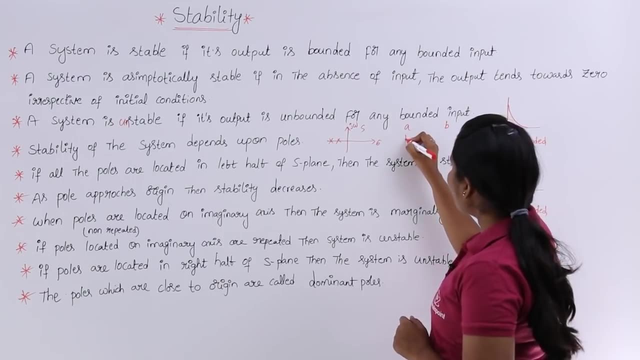 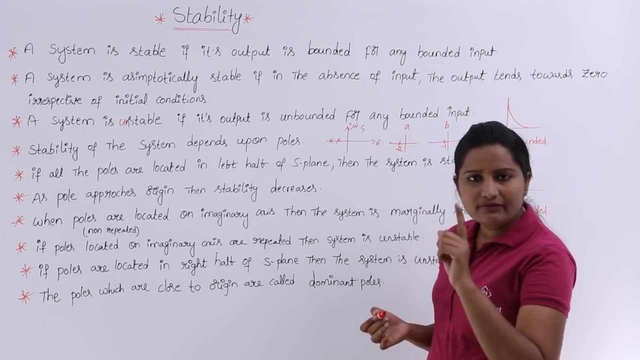 zero plot of the systems. you can say which system is much stable. For example, I am having system A and I am having system B. I got my pole zero plot. So here at minus 2 I am having pole and here at minus 1 I am having pole For system A. I am having only one pole at. 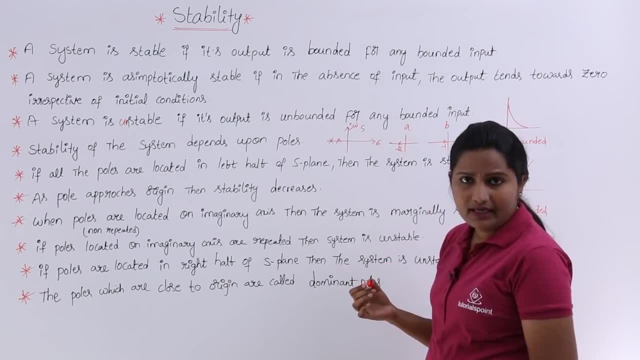 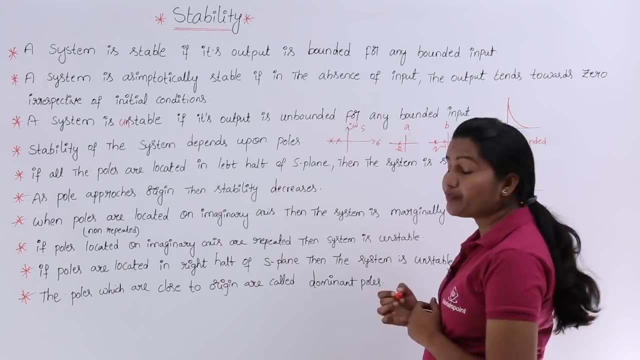 minus 2. and for system B I am having single pole at minus 1.. For example, here you are having minus 2.. Here, which system is much stable, means So this system is much stable. Why? Because here the poles are unbalanced. So here the poles are unbalanced. So here: 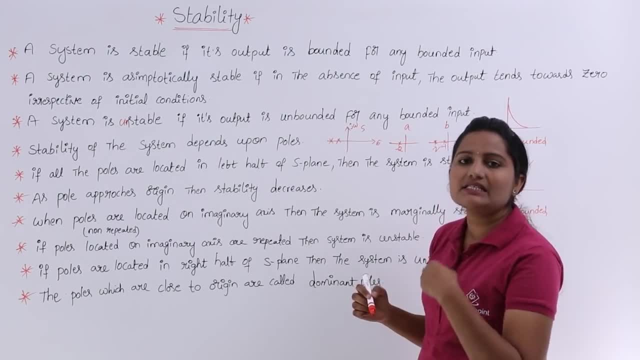 the poles are unbalanced, So where both of them are approaching origin, the poles of system B is very near to origin. If the poles are approaching to origin, the stability of the system will decrease. In these two systems, which system is more stable means? 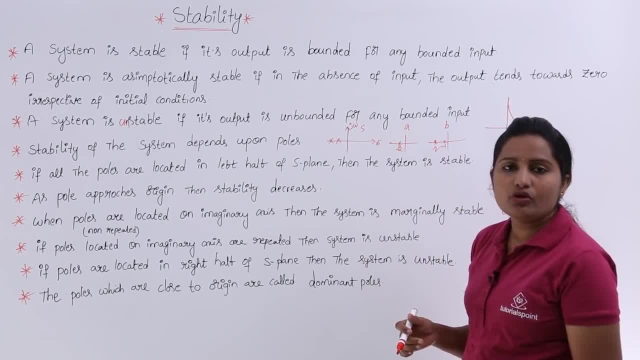 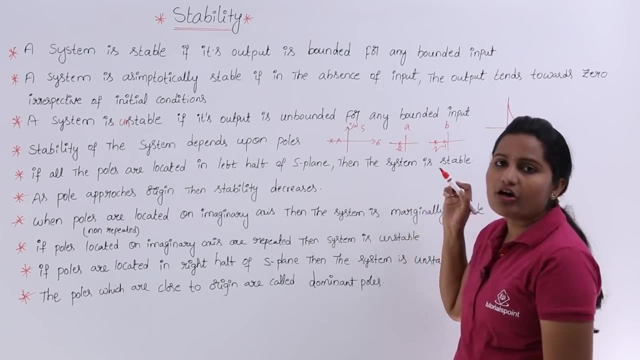 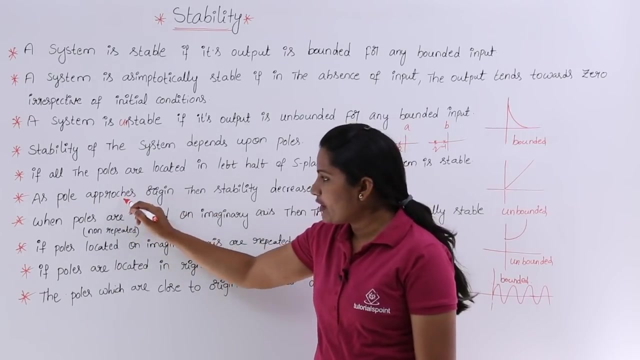 in these two systems. which system is more stable means A system is more stable because the pole of the system is more away from origin. so that is the reason. so, based on this point, based on this point, we can say we can justify the stability of the system. B is very stable. 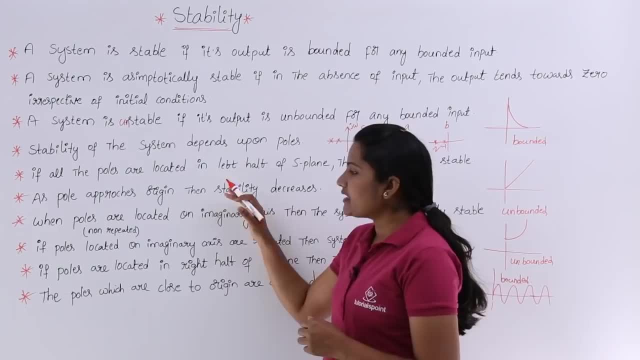 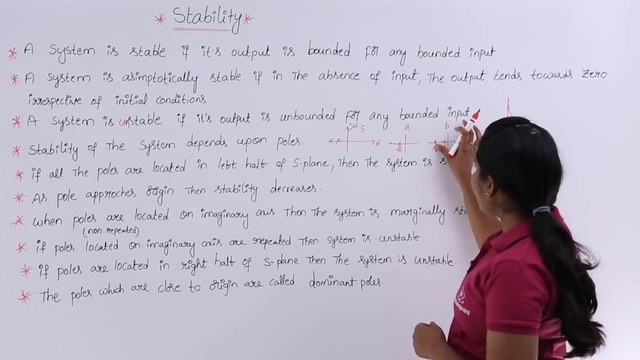 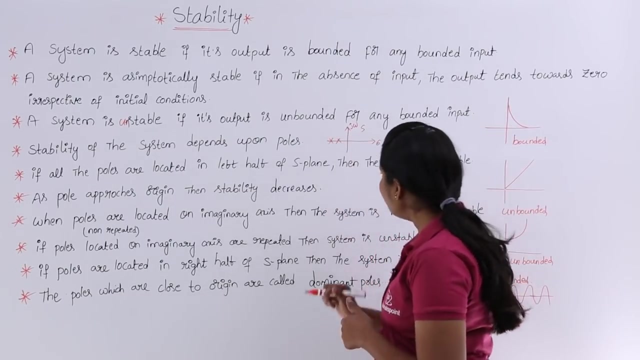 in system according to pole 0 plot and coming to this point, when poles are located on imaginary axis, for example, here you are having one pole like this. so here I am going to consider another diagram, another s plane. so if you are having s plane like this, this is j omega axis and 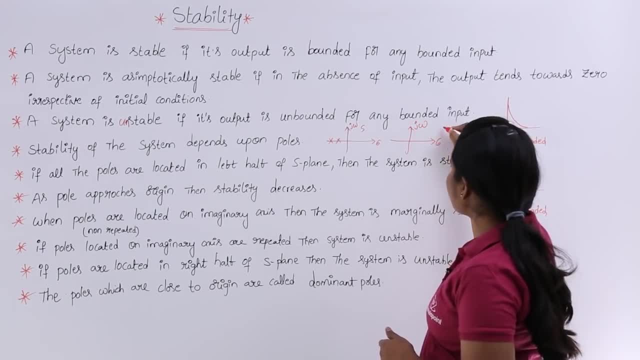 this is real axis, this is totally s plane. if your pole, if your poles are located one side is your pole, this is j omega and this is j omega the other. we can say: this is j omega or this is j omega, this is j omega k. 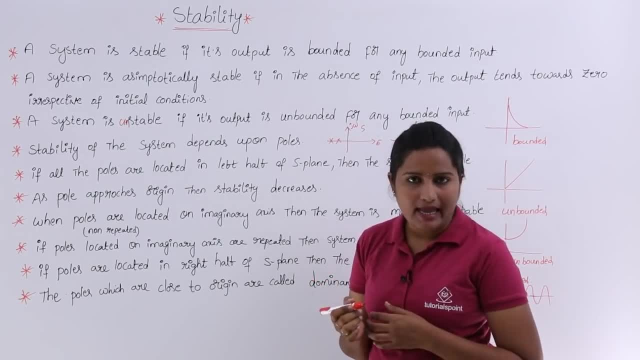 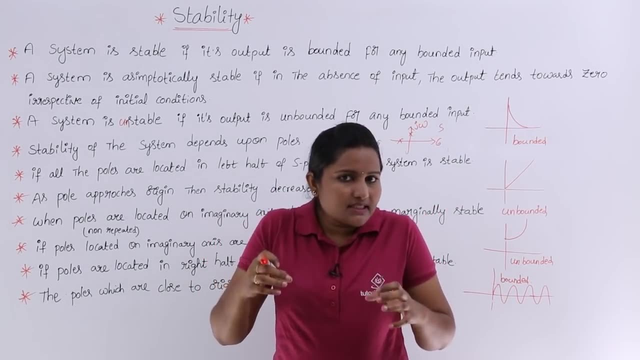 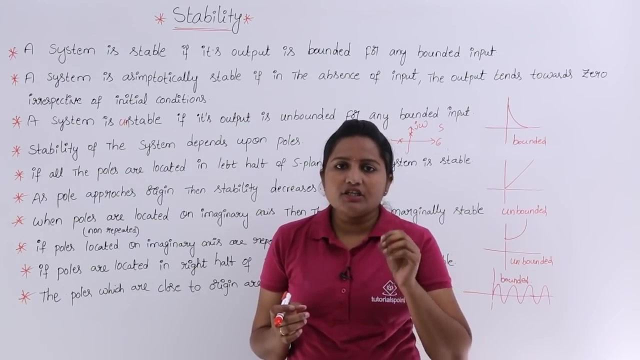 one of the pole, or some poles are located on imaginary axis, then we can say that is marginally stable system. In that justification of marginally stable system also, we need to follow one condition: Poles need to be on imaginary axis and non-repeated When the 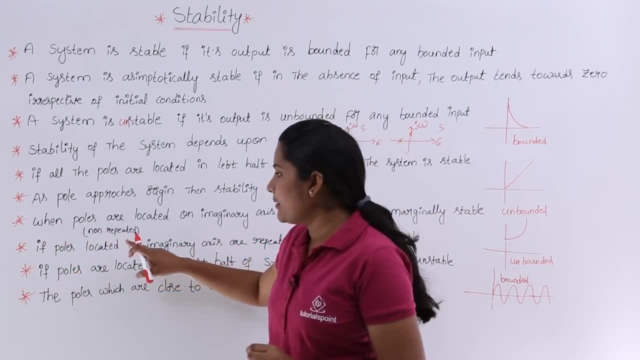 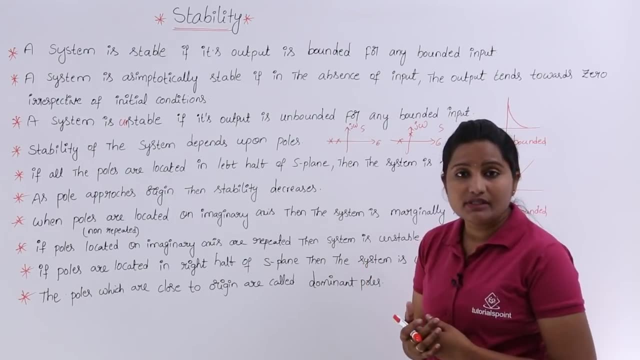 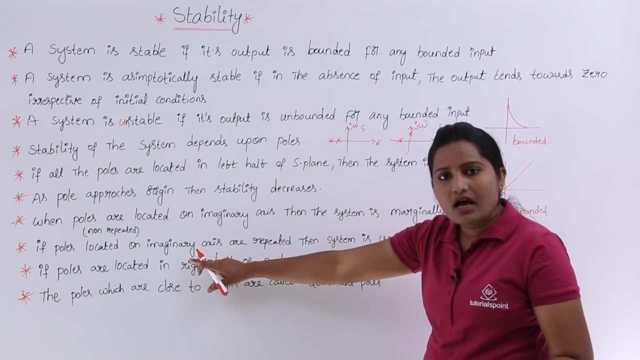 poles, or when the roots or non-repeated poles are located on imaginary axis, then the system is said to be marginally stable system, Whatever the poles located on imaginary axis. if that located poles are repeated poles, then we can say that is a unstable system. We cannot. 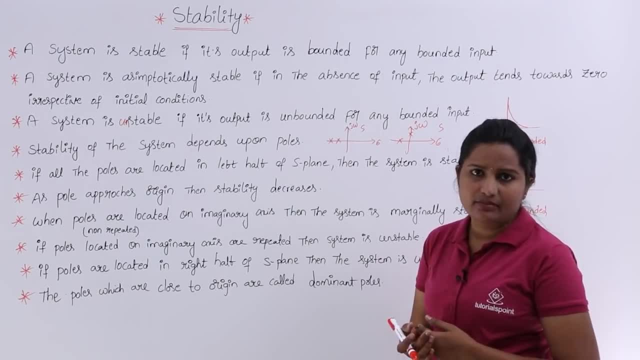 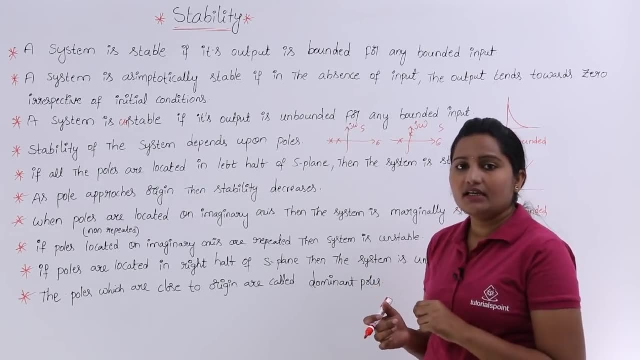 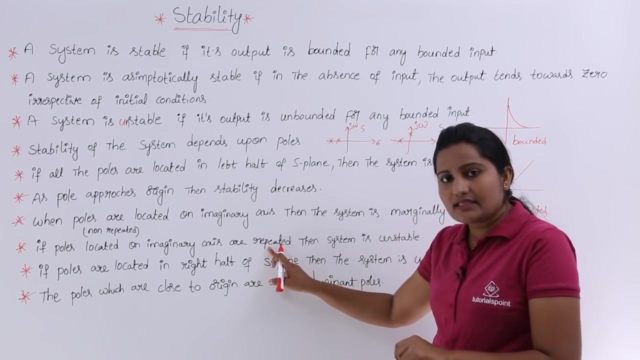 say that is imaginary, marginally stable system. If poles are located on imaginary axis and non-repeated, then only we can say that system is marginally stable system If poles are located on imaginary axis and repeated. when poles are repeated on imaginary axis. 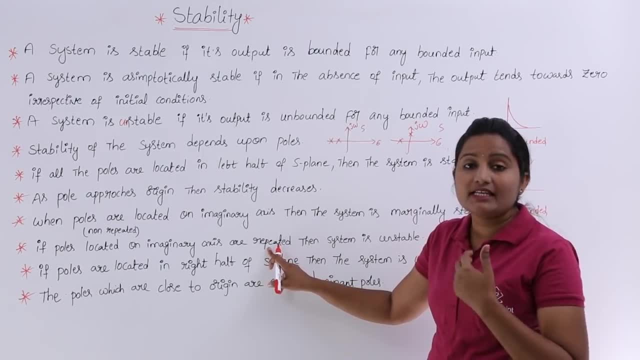 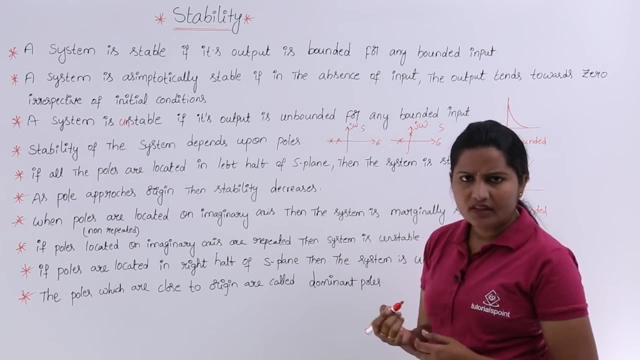 then definitely we cannot say that is marginally stable system. we can say that is unstable system. That means if you are having minus j and plus j repeated poles, then we can say that is unstable system, Thank you. So if different poles are located on imaginary axis, then we can say that is marginally stable. 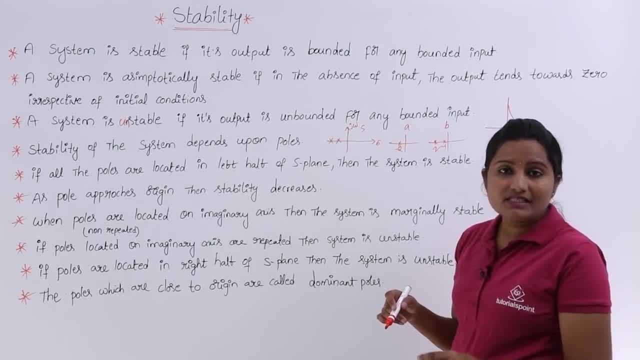 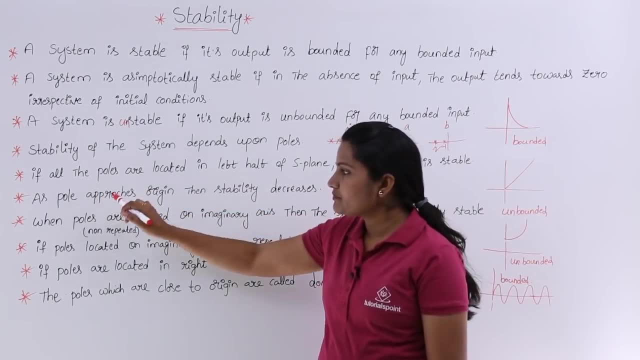 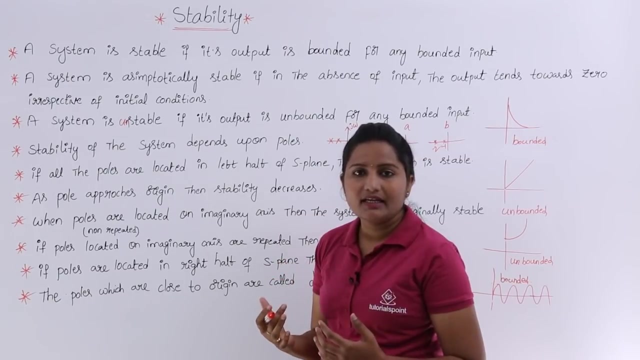 A system is more stable because the pole of the system is more away from origin. So that is the reason. So, based on this point base, drawn this point, we can say that this system A is very stable. say, we can justify the stability of the system according to pole 0, plot And coming to this, 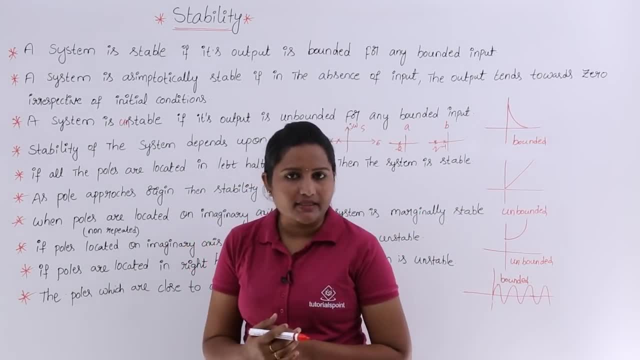 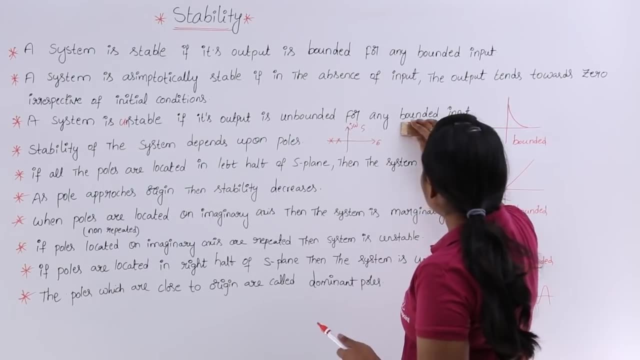 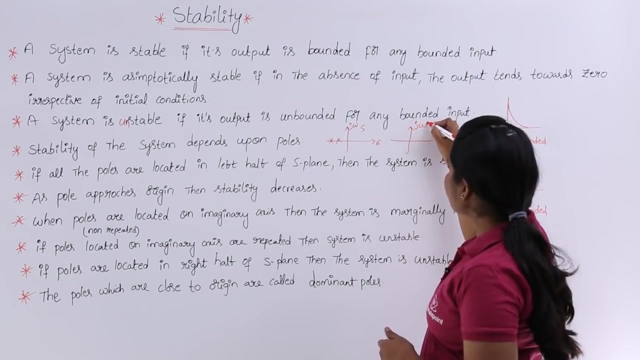 point when poles are located on imaginary axis. For example, here you are having one pole like this. So here I am going to consider another diagram, another S plane. So if you are having S plane like this, this is j omega axis and this is real axis. this is totally. 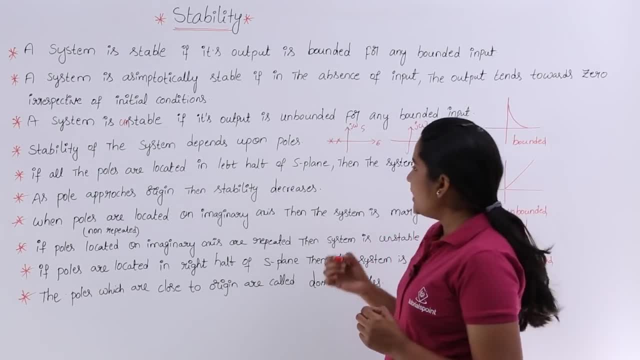 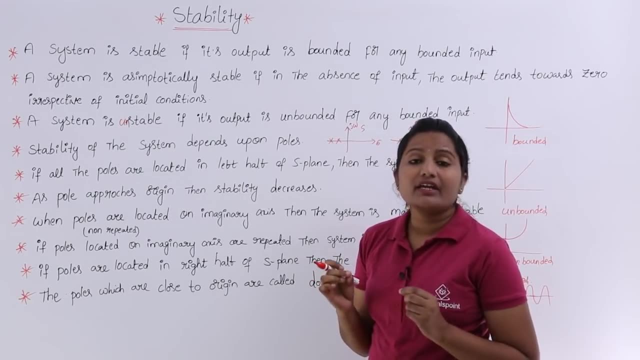 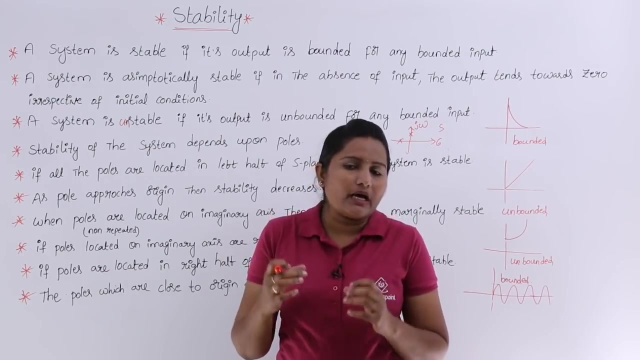 S plane. If your pole, if your poles are located one of the pole or some poles are located on imaginary axis, then we can say that is marginally stable system. In in that justification of marginally stable system, also, we need to follow one condition. 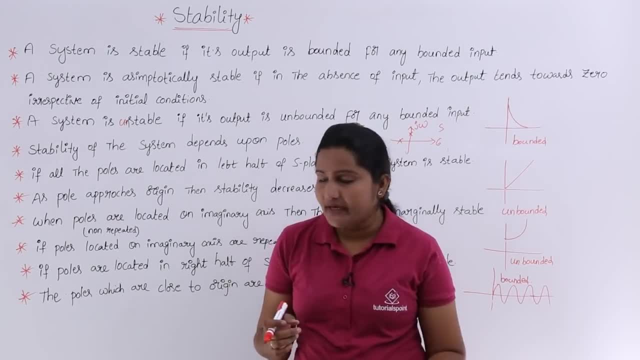 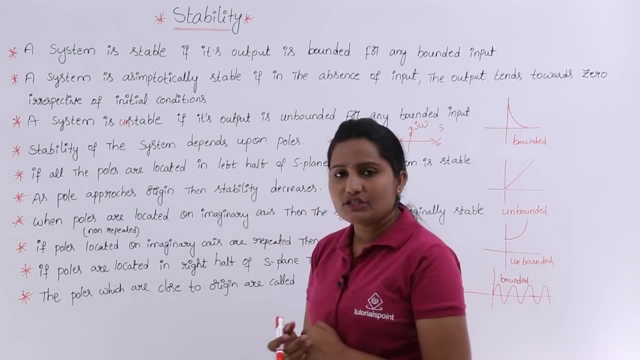 Poles need to be on imaginary axis and non-repeated When the poles or when the right and left side. if the poles et al, some poles, are on imaginary axis, If the poles, yours- are not effected surrounding the stalk and not located on imaginary axis, then these are repeated. 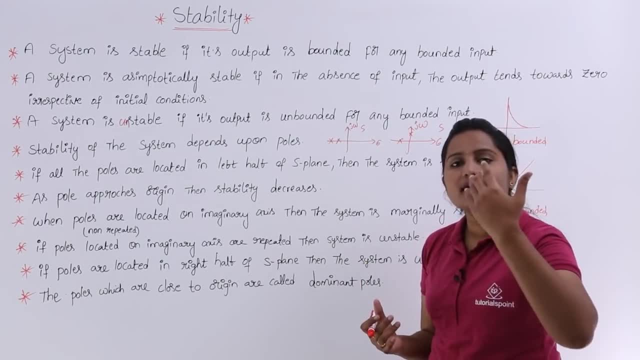 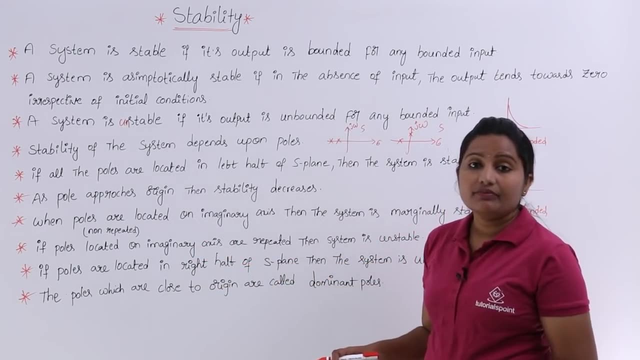 energy. that is that pole system And this is what is called as marginal stabilizing system. So if the poles are located in imaginary axis, then this system is said to be a argument controlling the imaginary position of the pole. Now, on imaginary Links, it is in wraps. 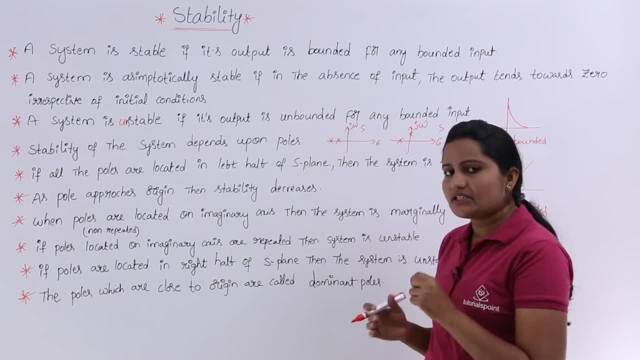 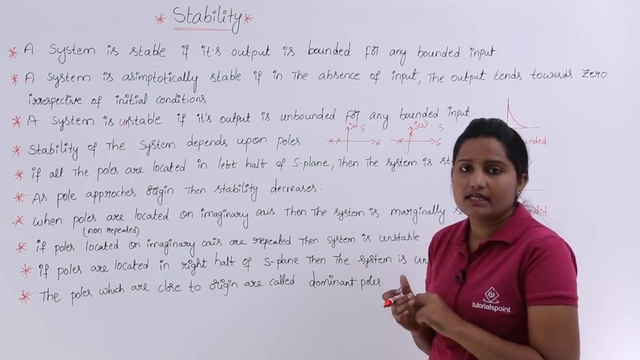 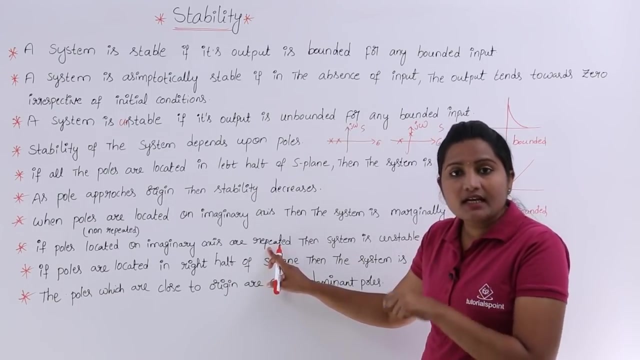 when the poles are took and arched Again- original according to there is relocated long and non-repeated- then only we can say that system is marginally stable system if poles are located on imaginary axis and repeated. when poles are repeated on imaginary axis, then definitely we. 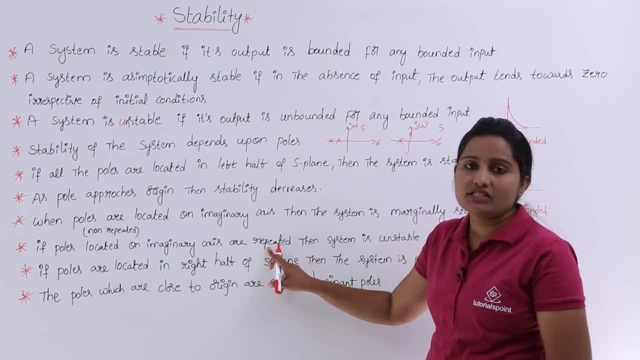 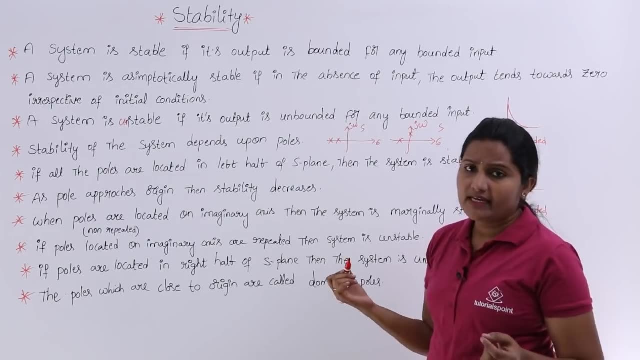 can't say that is marginally stable system. we can say that is unstable system. that means if you are having minus j and plus j repeated poles, then we can say that is unstable system. so if different poles are located on imaginary axis, then we can say that is marginally stable system and definitely. 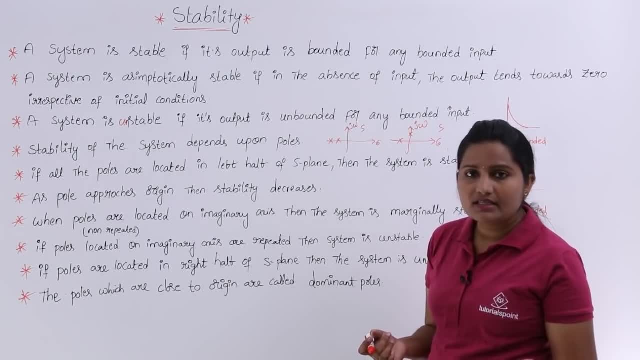 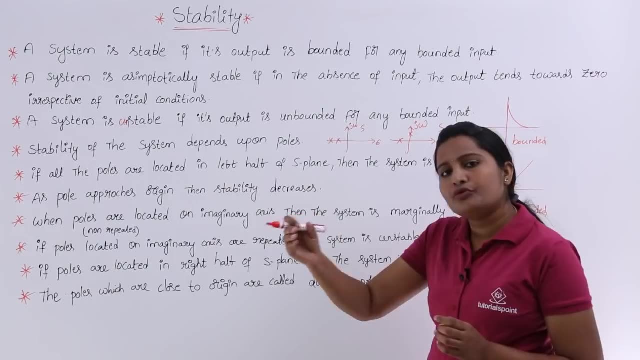 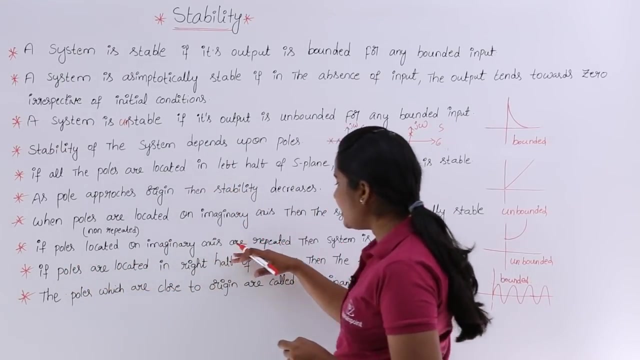 system and definitely the remaining poles. if is there any remaining poles, then that should be on left half of S plane. If at least one pole moved to right half of S plane, definitely we can say that is unstable system. If poles located on imaginary axis are repeated, then 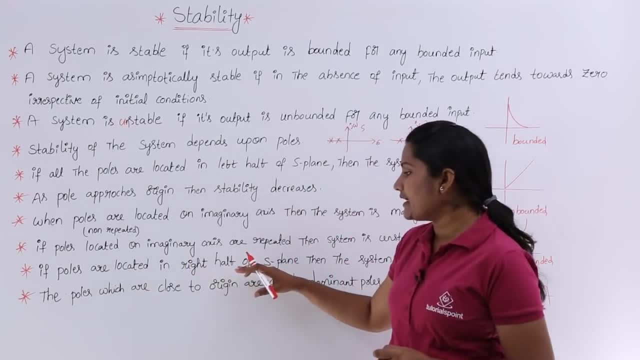 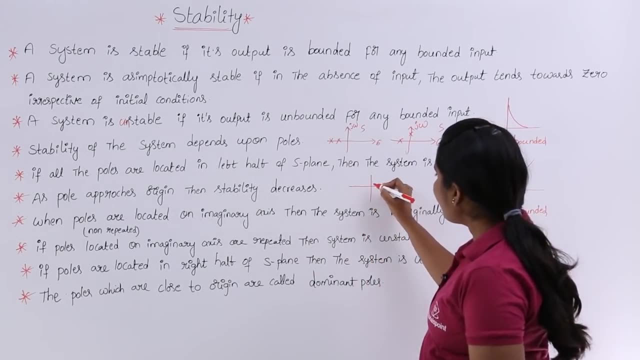 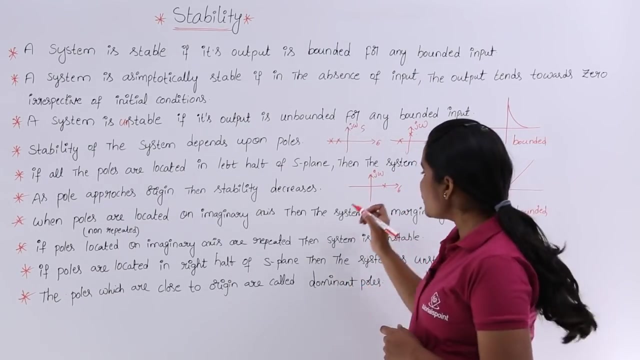 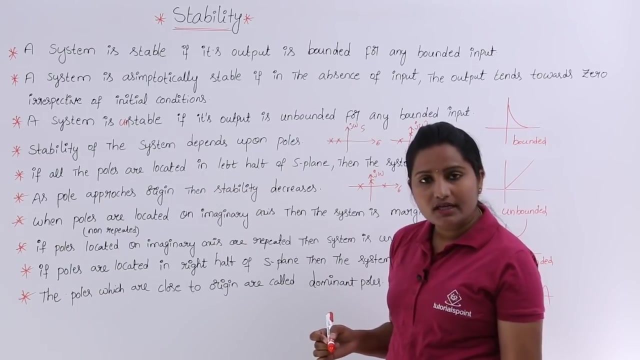 the system is unstable. If poles are located on imaginary axis, then we can say that is non-repeated because there are few Random getting rising and falling poles. So we can say that if poles are located on imaginary axis and repeated, then we can say that is unsustainable and it clearerıyor. 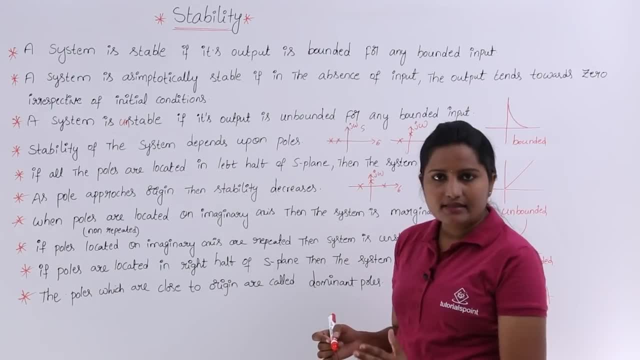 Same thing equal to 0.. OK, So if poles are located on imaginary axis and repeated, if poles are located on imaginary axis, we can say: that is Gavin 0.. neo1 complex patient. Well, Did you understand That is true? Yes, Just here also we can say that is correct because S plane is till there. 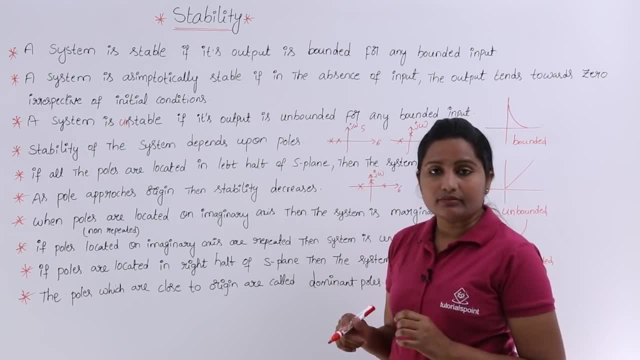 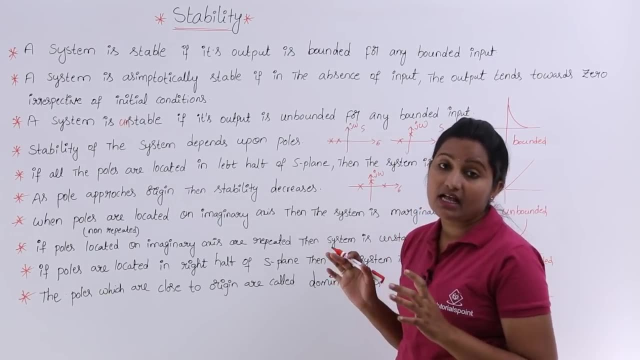 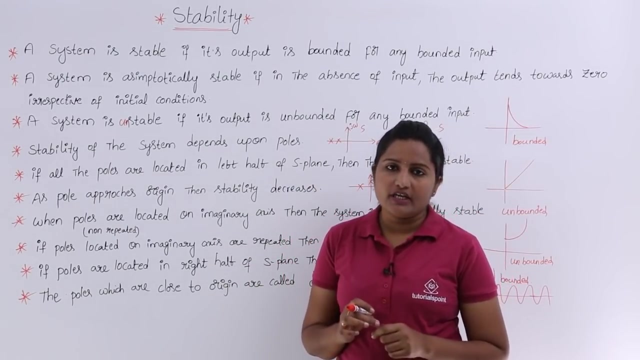 then also this is unstable system. That means if at least one pole shifted to right half of S plane, we can say that is unstable system. So like this, we will define the stability of the system according to pole locations. poles will define the stability of the system. 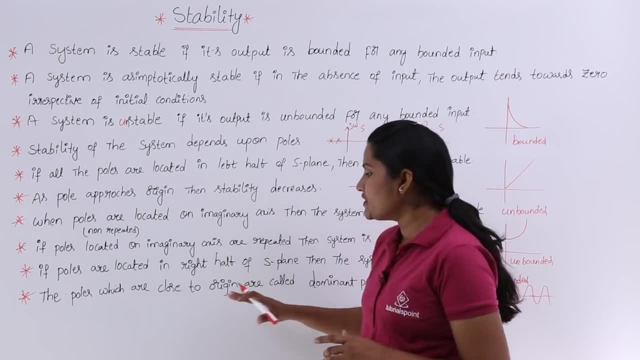 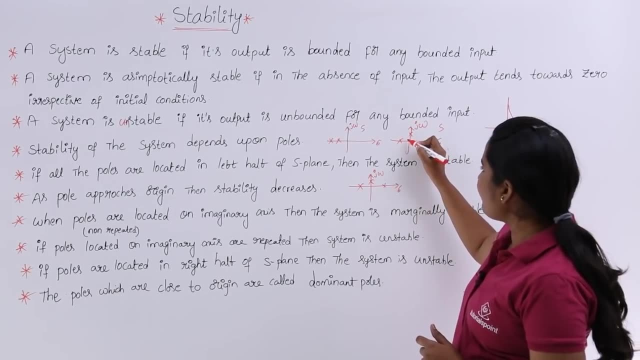 So, coming to the last very important point, the poles which are close to origin are called as dominant pole. So here, for example, here you are having some, I am having pole 0 plot like this: j, omega axis and real axis and minus 1 and minus 2 or 2 poles I am having in the 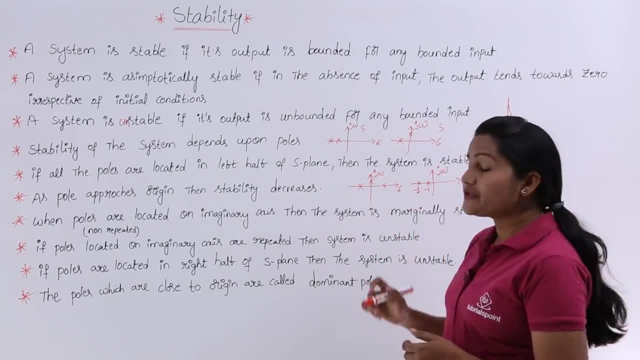 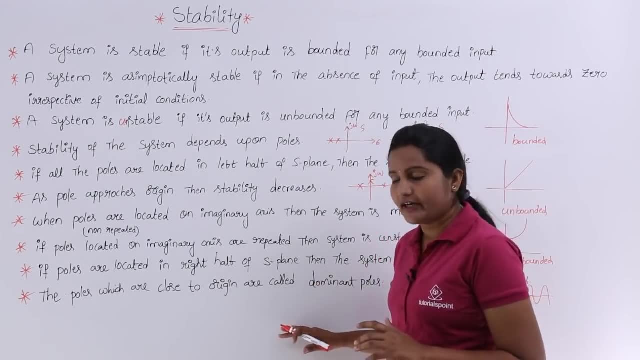 left half of S plane. So here, in these two poles, which is the dominant pole, means minus 1 is the dominant pole. how we can say, means: according to this point, The poles which are very close to origin are called as dominant pole. So here, in this two poles, which is: 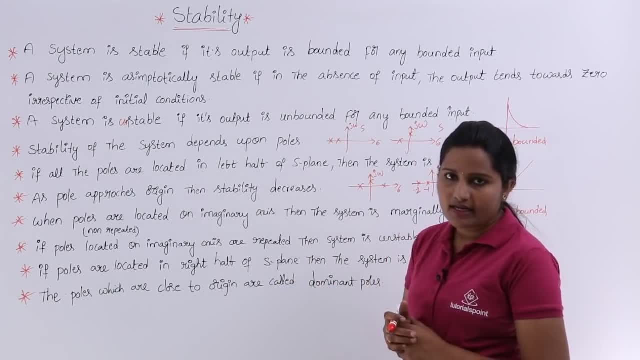 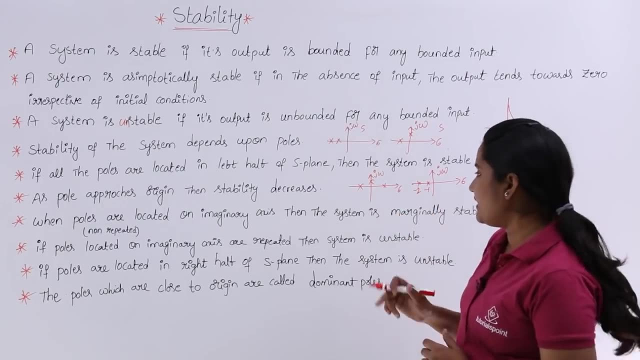 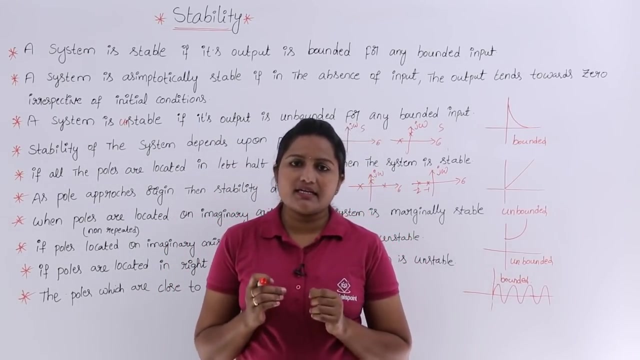 close to origin are 0 is are called as dominant poles. So here minus 1 is the dominant pole than minus 2.. So this is about introduction for stability. So stability is nothing, but generally you need to get bounded output for bounded input. 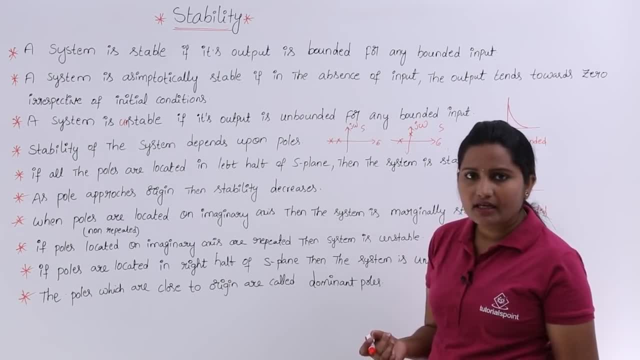 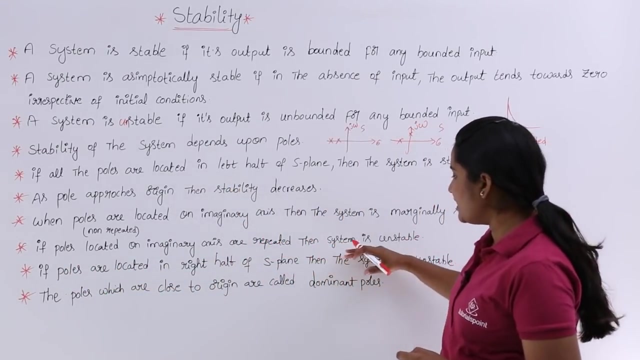 the remaining poles? if is there any remaining poles, then that should be on left half of s plane. if at least one pole moved to right half of s plane, definitely we can say that is unstable system. if poles located on imaginary axis are repeated, then the system is unstable. if poles are located. 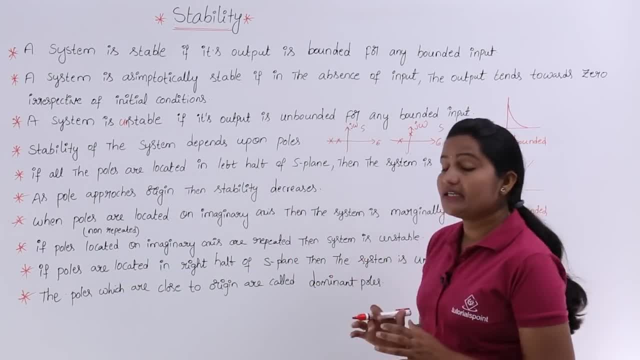 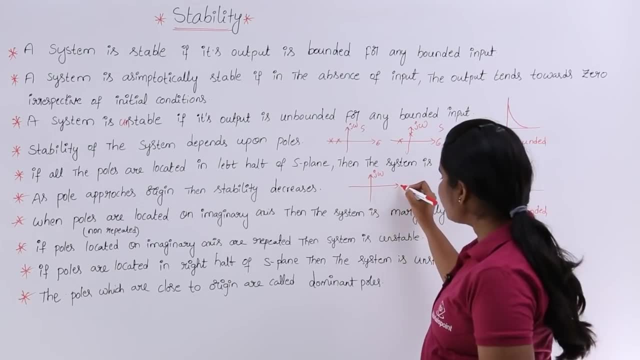 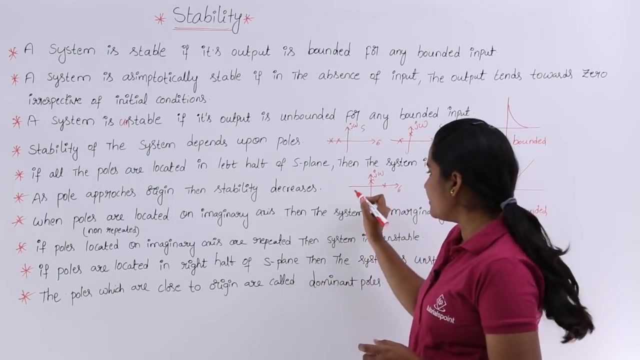 in right half of s plane, then the system is unstable system. that means, for example, if you are having poles like this j, omega and sigma, if you are having like this unstable system. so if you are having poles like this unstable system, if you are having three poles, one pole is located. 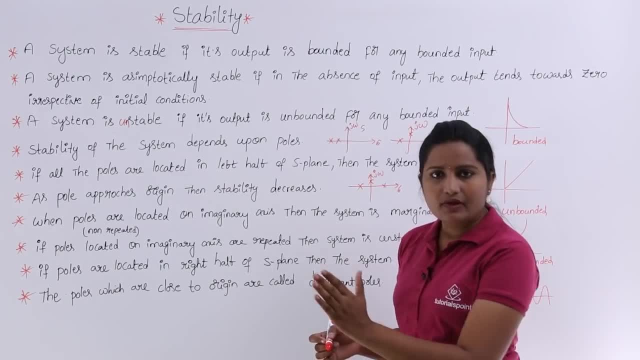 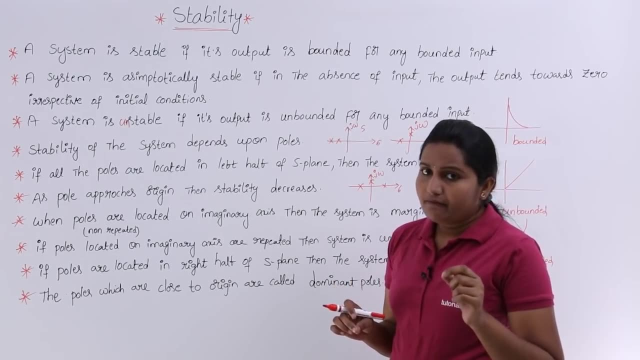 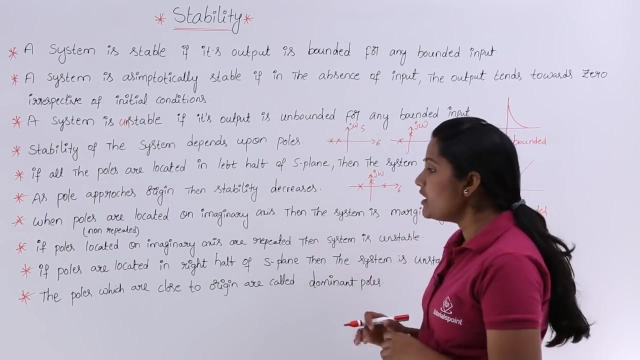 left side of s plane, one is imaginary axis, one is right half of s plane, then also this is unstable system. that means if at least one pole shifted to right half of s plane, we can say that is unstable system. so like this we will define the stability of the system according to pole locations, poles. 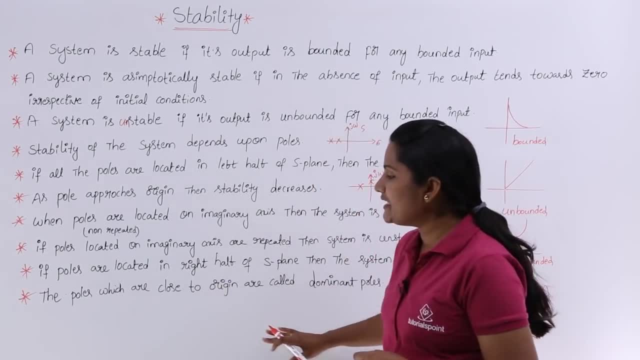 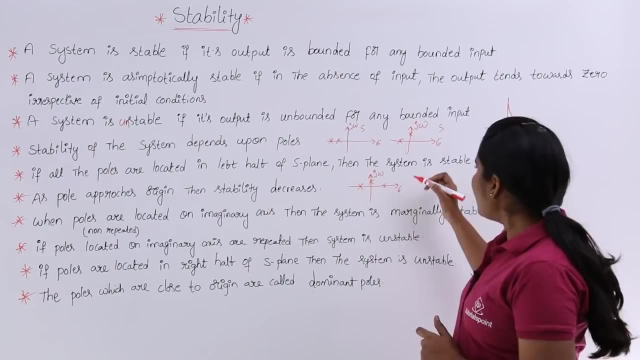 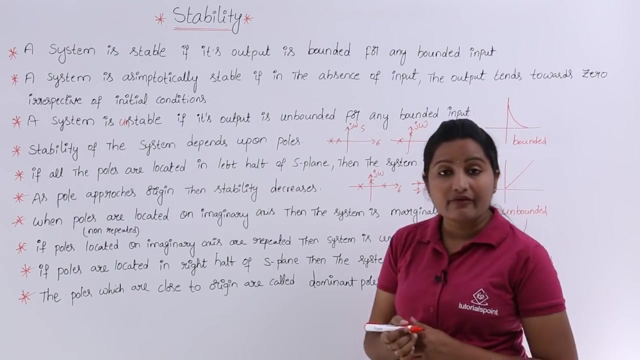 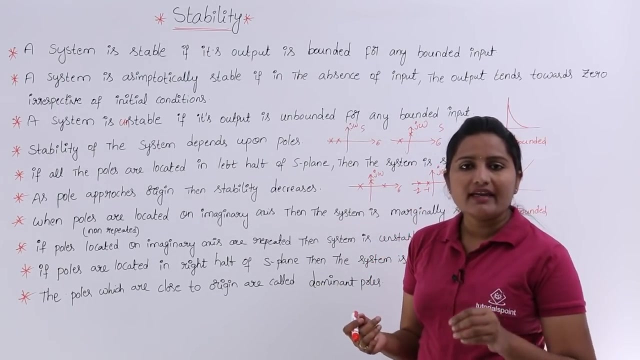 will define the stability of the system. so, coming to the last very important point, the poles will have a dominant pole. Now we can see that. so here, in these two poles, which is the dominant pole means minus 1 is the dominant pole. How we can say that? 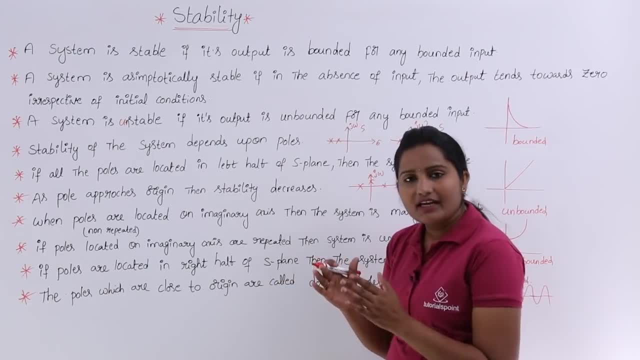 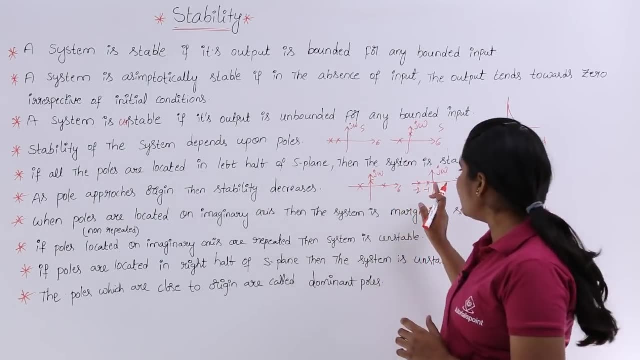 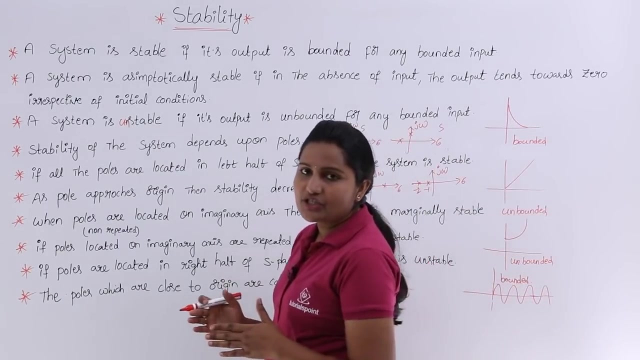 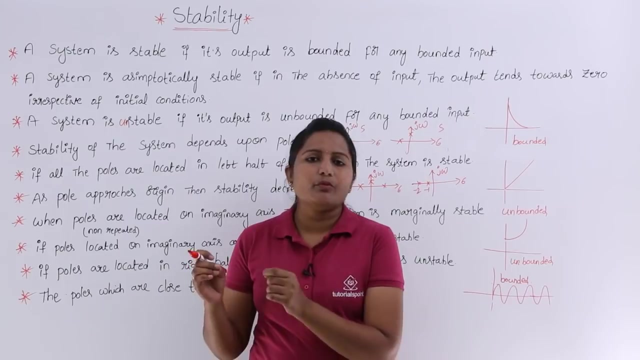 same is. according to this point, The poles which are very close to origin, or 0 is, are called as dominant poles. So here minus 1 is the dominant pole than minus 2.. So this is about introduction for stability. So stability is nothing but generally you need to get. 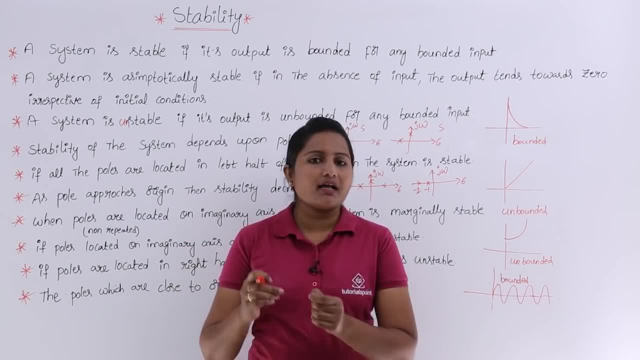 bounded output for bounded input. If you are getting unbounded output for bounded input, that system is said to be unstable. So here bounded signal is nothing. but the finite values must be there. that means the maximum and minimum value of the signal must.